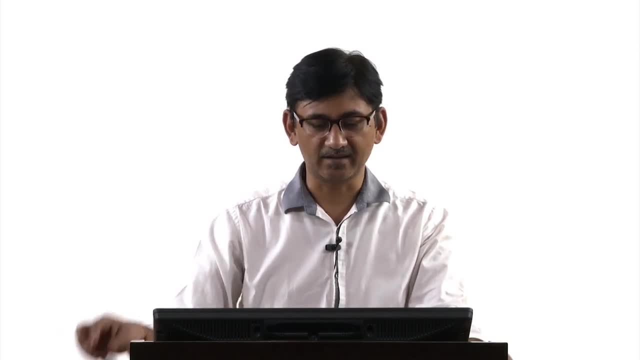 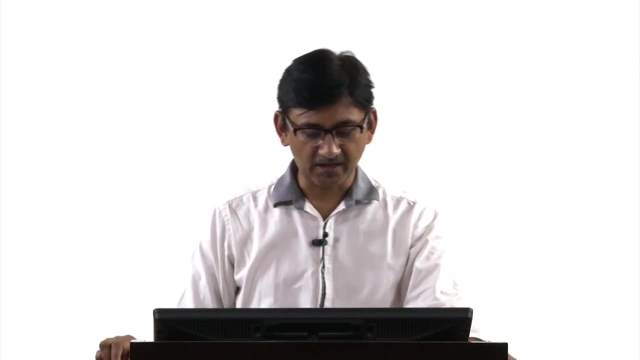 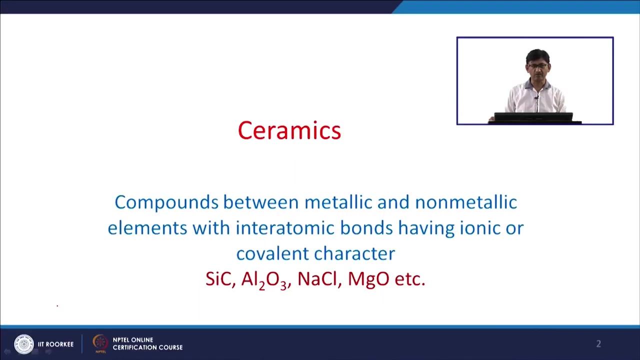 materials are the most widely used material and these materials are used in very specific applications. So ceramics are basically compounds between metallic and non-metallic elements with inter atomic bonds having ionic or covalent character. So, for example, one of the very important ceramic material you might have come across. 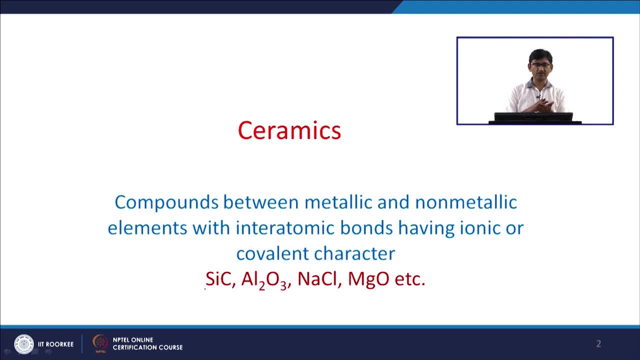 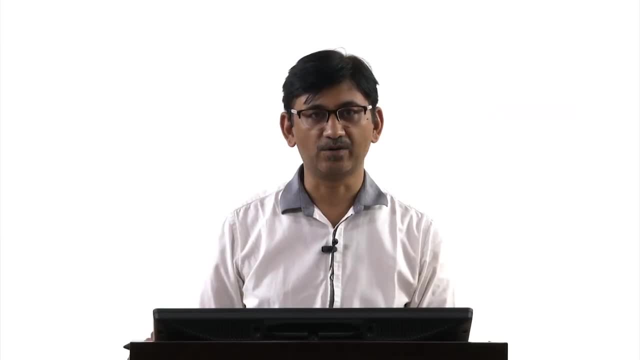 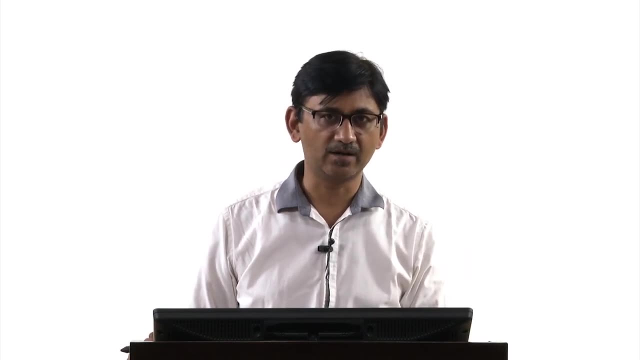 is silicon carbide. So in all your abrasive paper which you use for doing polishing or you must have seen. if any painter is coming to your home and he is rubbing the surface of the wall, May not be. they may not be using silicon carbide. 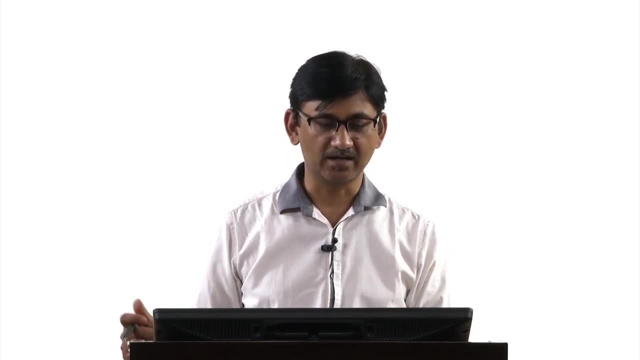 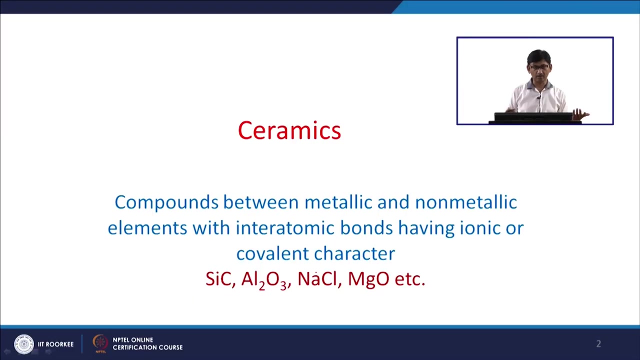 papers, but in the abrasive papers silicon carbide is one of the important ceramic which is used for abrasive application. Another class is aluminium oxide, Al2O3 sodium chloride. of course you must have used this is our common salt- and magnesium oxide. these are some few. 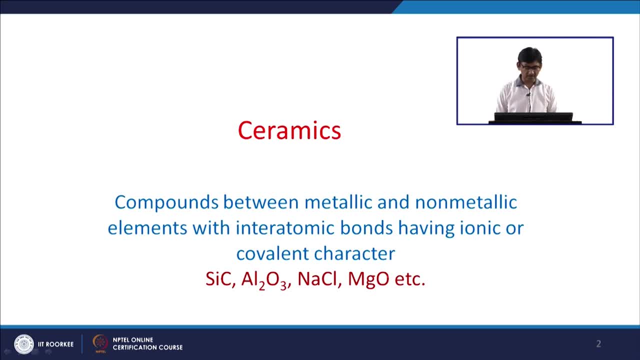 examples of ceramic materials. So in this case you can see that one of the element is a metal, another element is a non-metal and they both combine. So either they can have a covalent bond between them or they can have a ionic bond between. 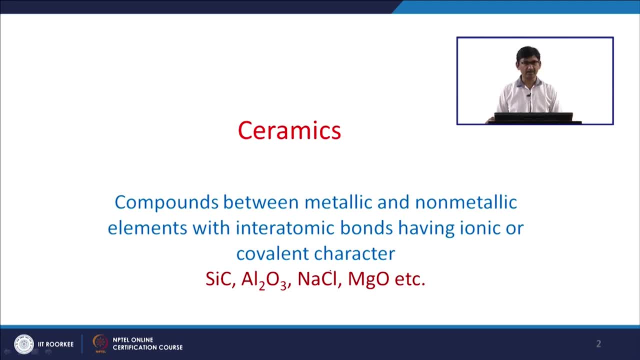 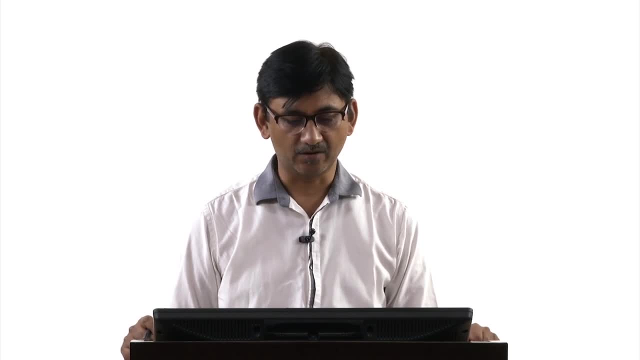 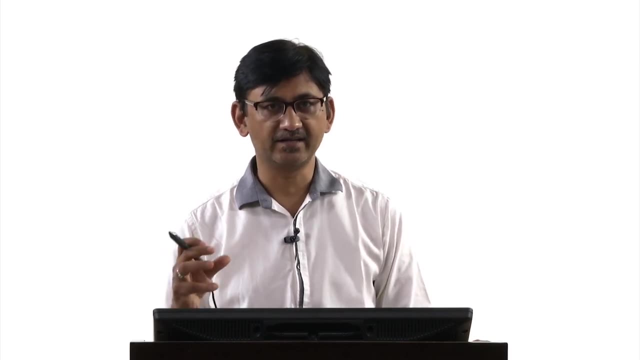 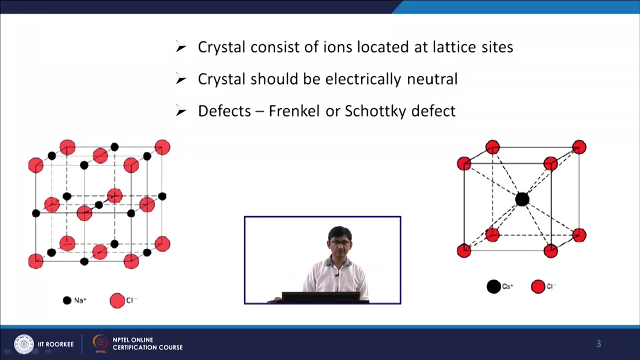 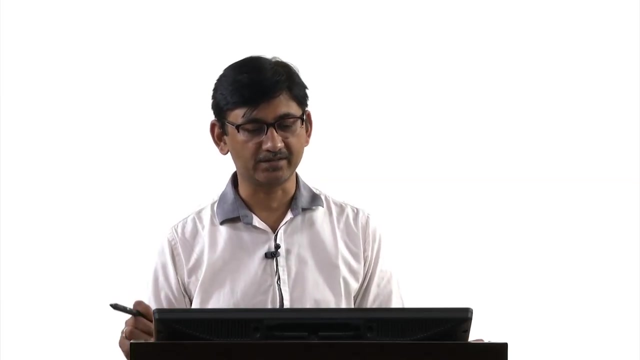 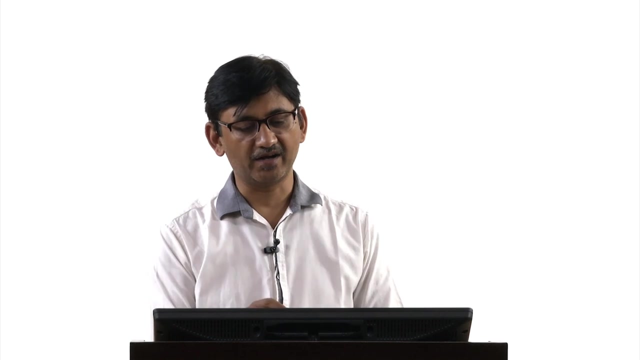 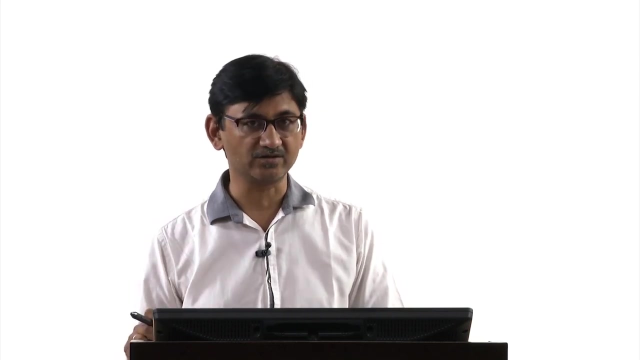 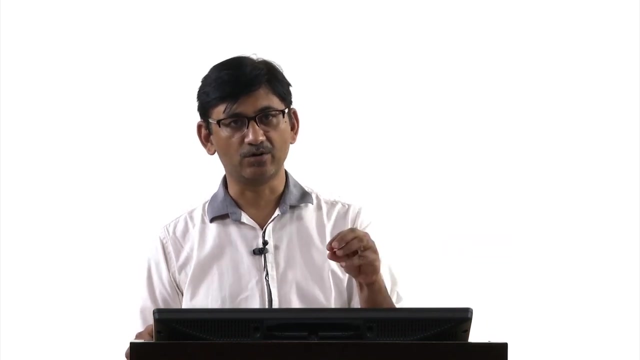 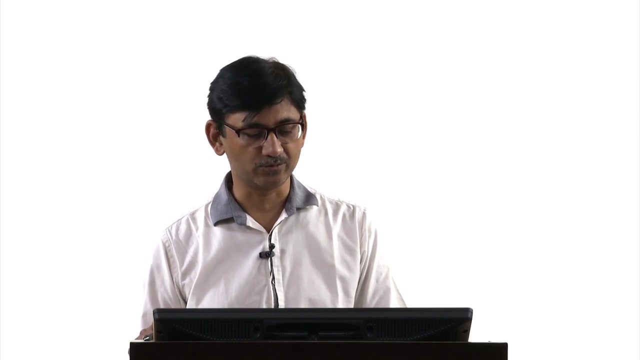 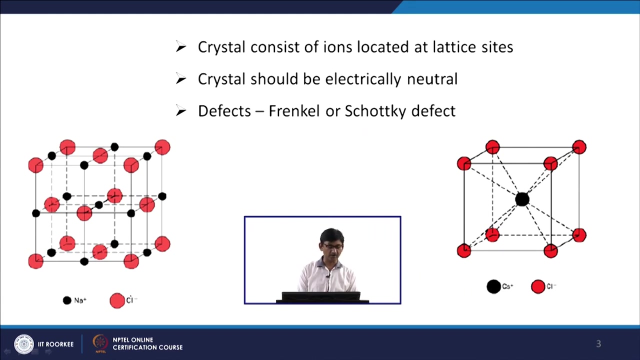 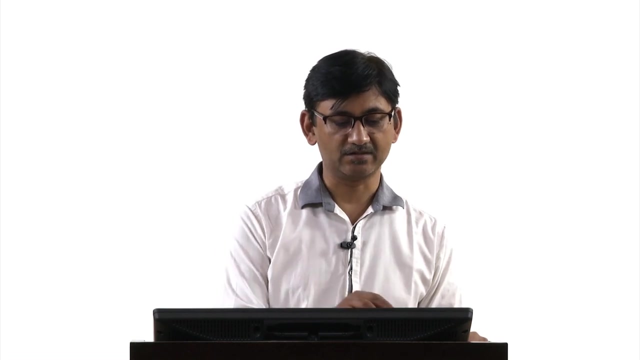 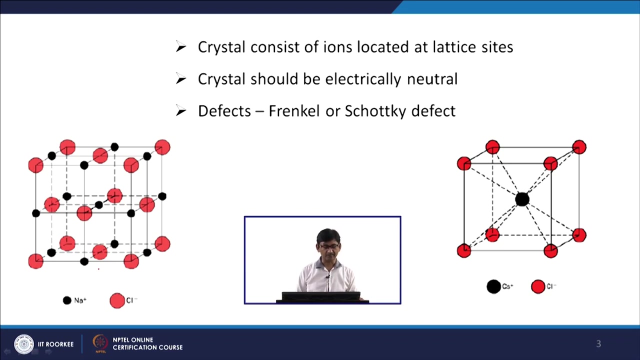 them and of course that is what affects their mechanical property to large extent. So just to have some idea about the crystal structure, So crystal consist of basically ions located at lattice sites. So this is the sodium chloride is based on FCC structure, two intervening FCC structure. 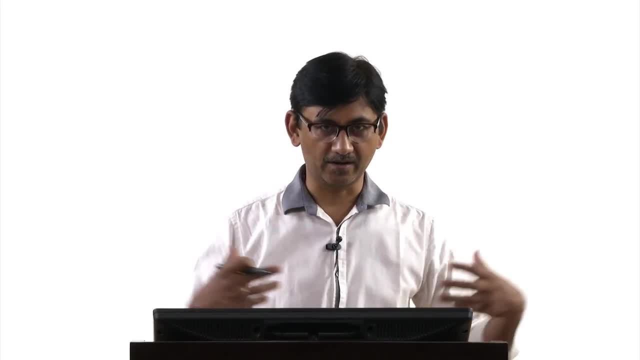 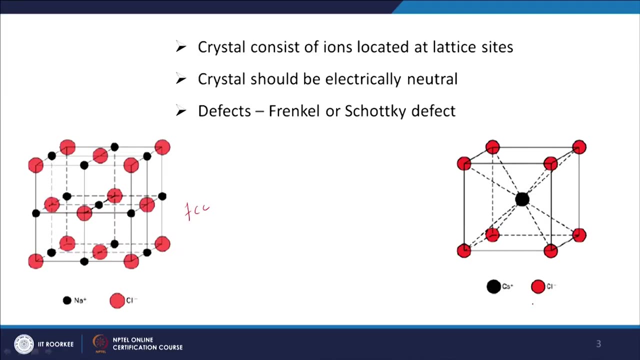 one for sodium, one for chlorine, and you can put them together to make a sodium chloride crystal. This is for a cesium chloride, another type of structure based on another known crystal structure which is known to us. This is based on BCC system. So you can see, one chlorine atom is at the centre of 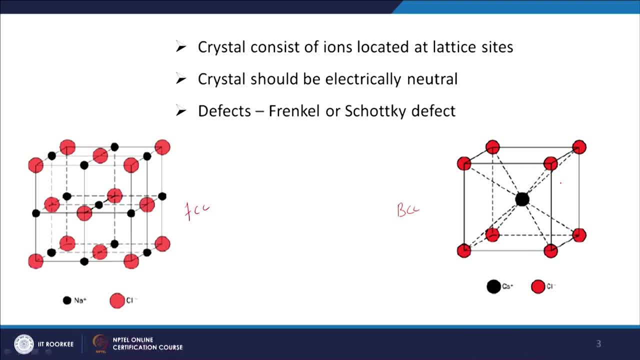 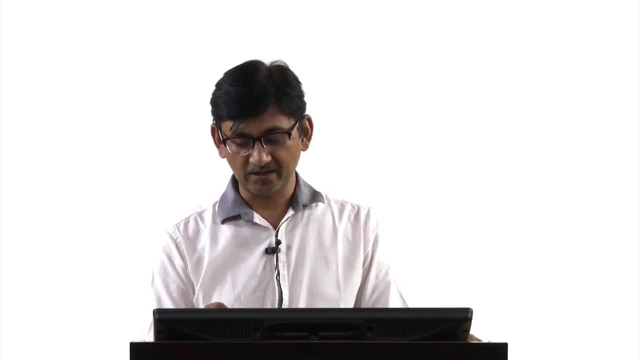 this BCC cell and there are a chlorine cesium atom, a chlorine atom at the at the corners. ok, Now, in looking that this unit cell, you might think that there is. no, you cannot maintain a electrical neutrality here. but if you see the BCC is position here is actually can be. 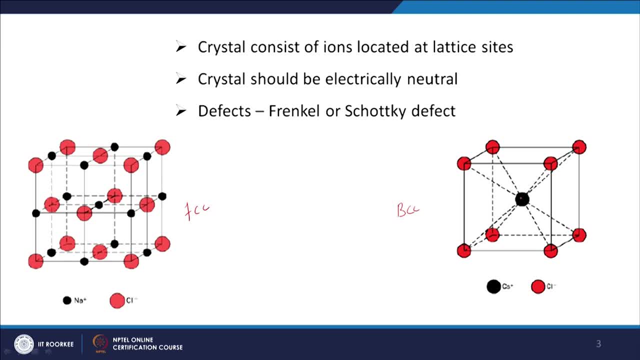 considered as a end position for another crystal. So if you make another crystal here, these cesium atom can be occupying the or another unit cell where cesium atom, the ions, are occupying the this end positions, and then you can see that chlorine will become the. 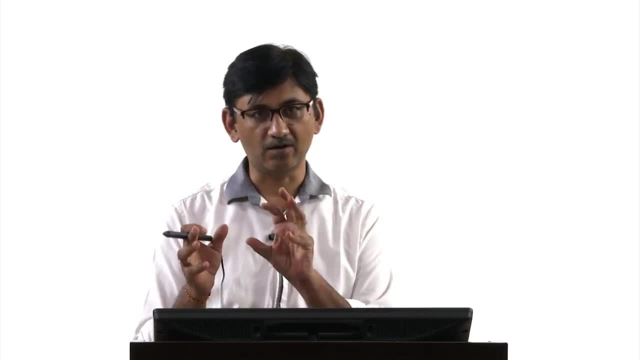 body centred one: ok, So these are all interchangeable. the centre atom in the body centred position, ok, can be. 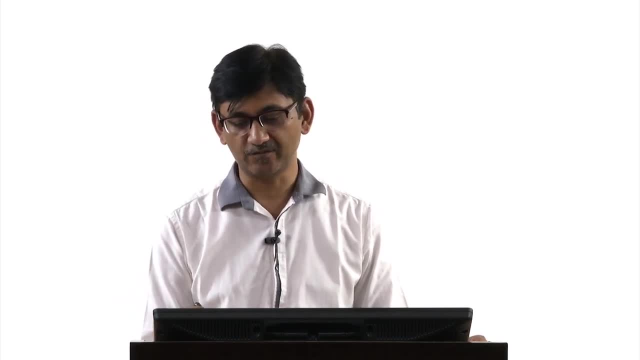 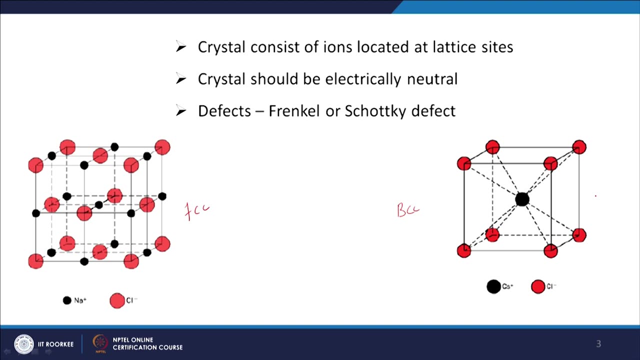 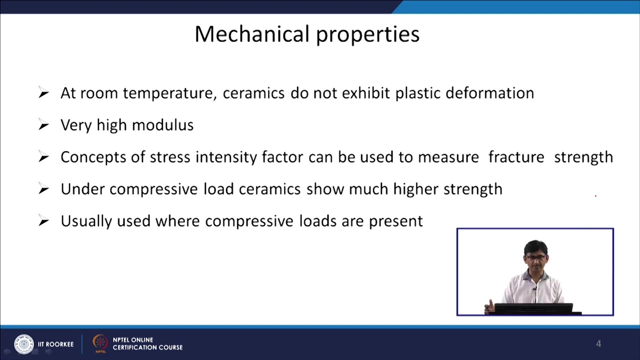 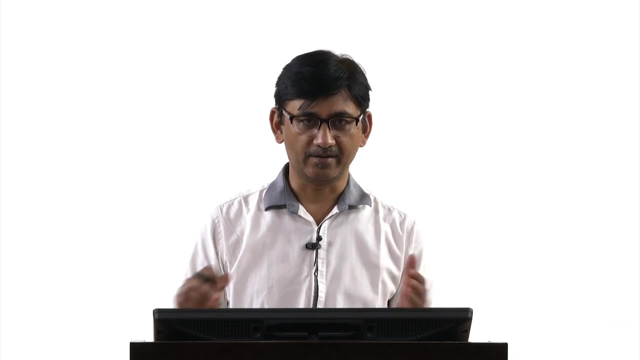 become a, become a corner position for another unit cell which you can make. So in overall, if you see, the electrical neutrality will be maintained for the whole crystal. The mechanical properties at room temperature ceramic do not exhibit plastic deformation. So basically they only show the elastic deformation part and then fracture. ok, 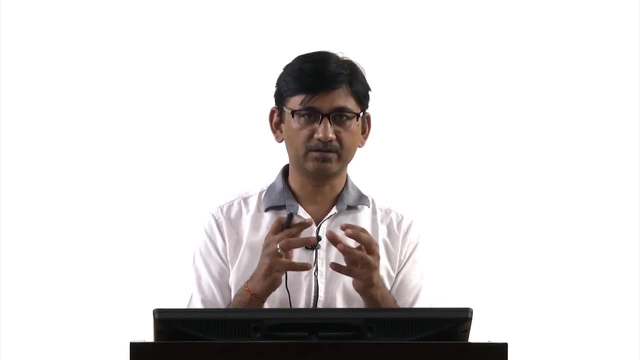 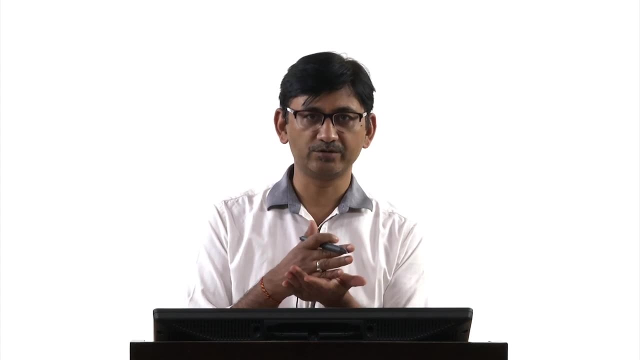 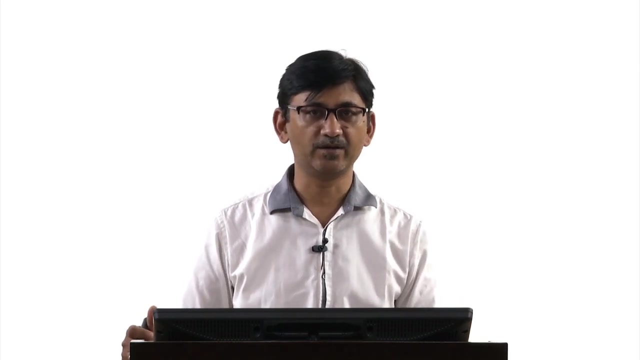 One main thing is the nature of the bonding. because they have covalent or ionic bonds, ok, They. the dislocation cannot be introduced here because that will bring an additional ion at the end- ok, and that will not be. we will not be able to maintain the charge neutrality. 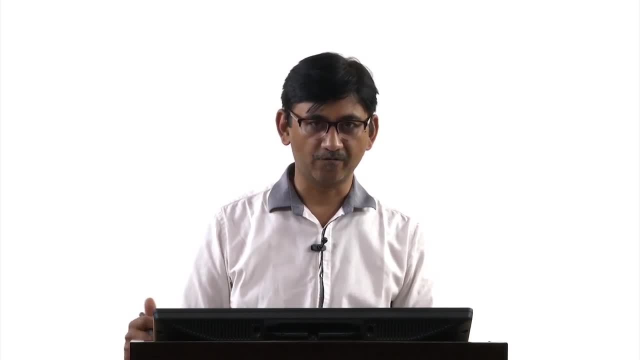 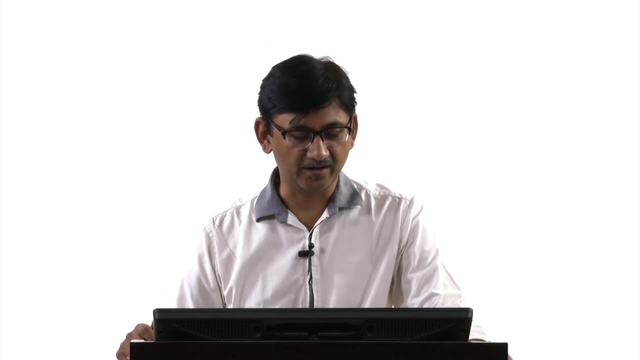 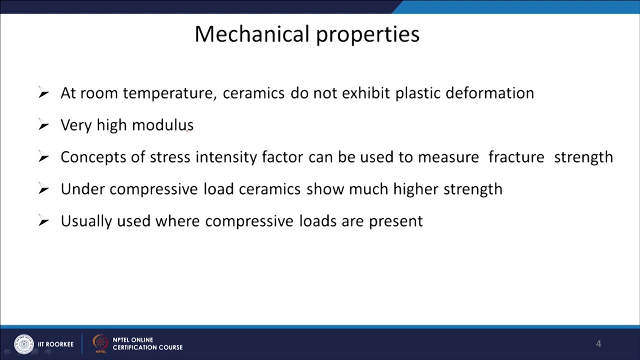 there, ok, So the deformation here is not, cannot be through dislocation movement and that is why the ceramics, So they are relatively failed without any plastic deformation, although they have very high modulus. ok, elastic modulus values are very high for ceramics. The concepts of stress intensity factor which we discussed when we were discussing fracture- 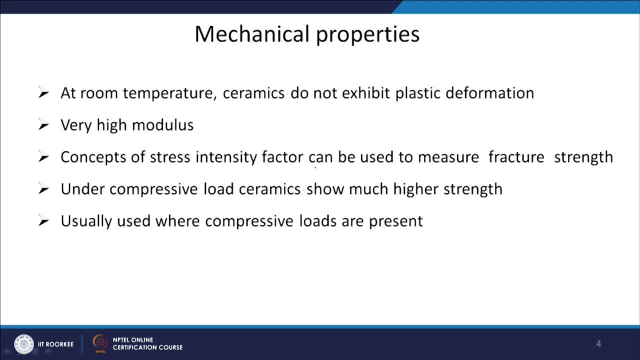 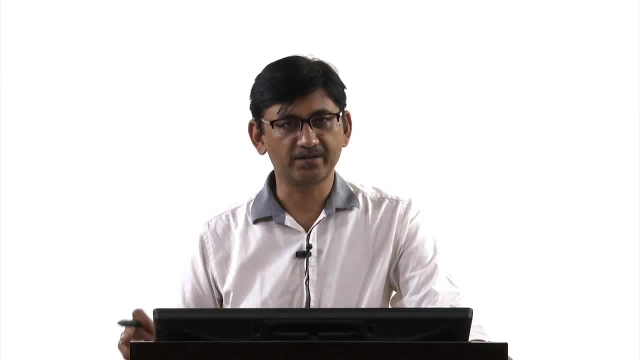 ok, can be used to measure fracture strength in the case of ceramics. ok, So because, again, the failure is through because of the defects which are present in the ceramic material And in form of a small cracks Or Or any flaws. and basically, when you apply any stress, they propagate and your material 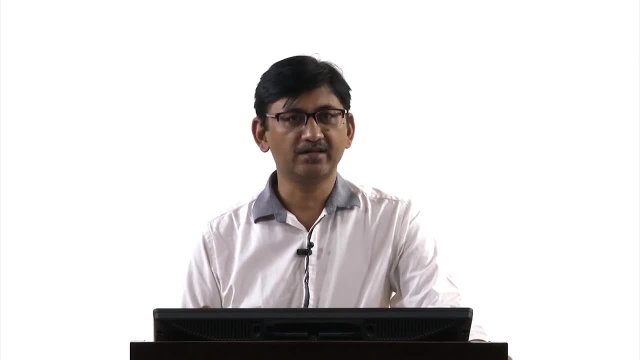 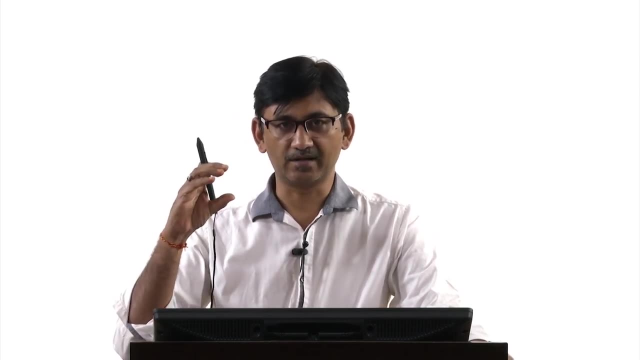 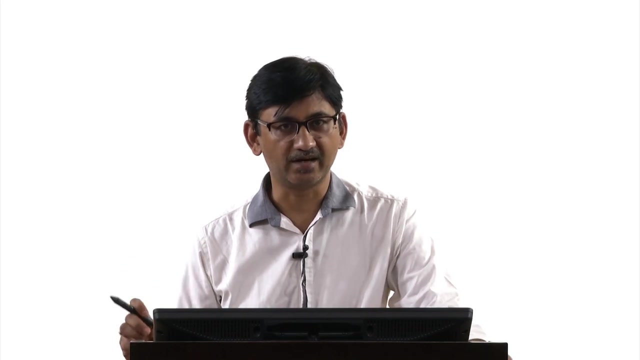 fail Under compressive load. ceramics show much higher strength. ok, They are able to take compressive load very nicely because in the compressive load your cracks do not open up. in fact you are closing them. ok, So ceramics can be used very nicely under compressive loading condition. 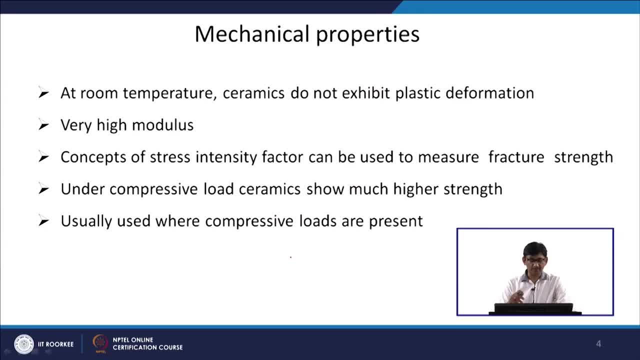 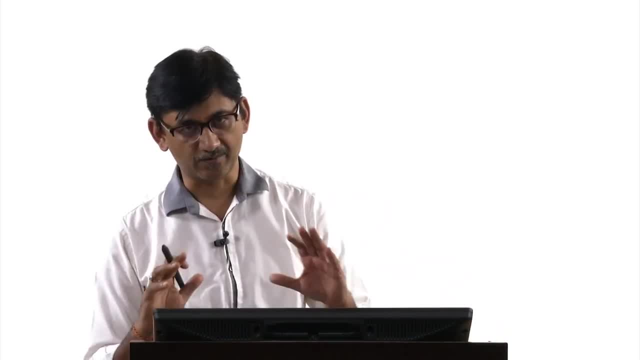 So that is why they are used where compressive loads are present. Ok, Measurement of properties: ceramics are not subjected to tensile test. ok, So the property measure or property evaluation in case of ceramics is not cannot be done through tensile test. ok. 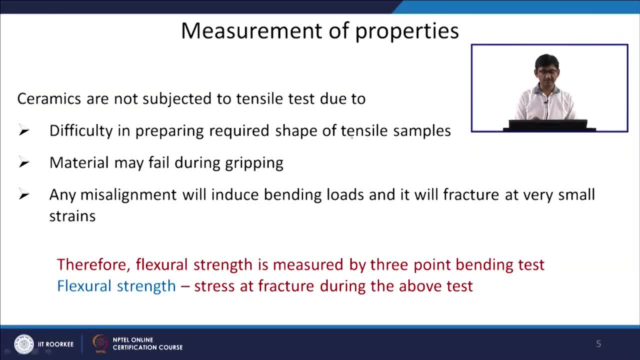 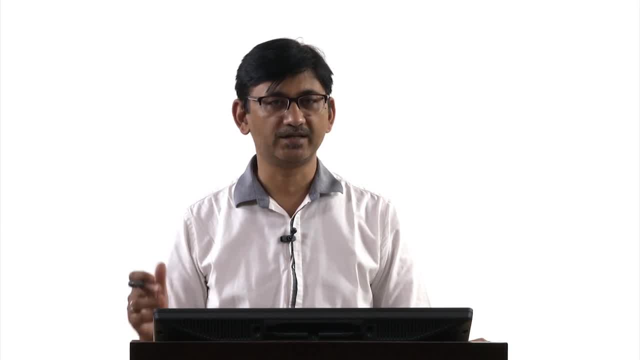 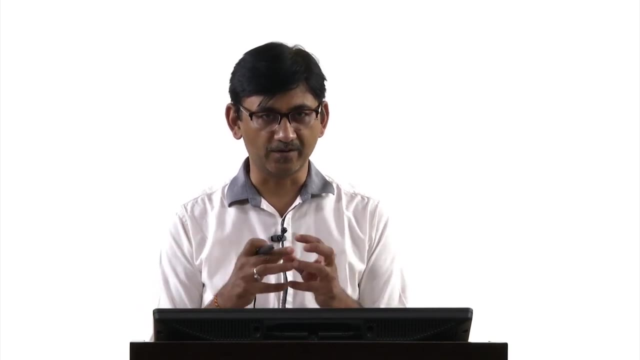 The reason is, first, is the difficulty in preparation which is required to create that shape of the tensile sample which we discussed earlier. ok, That what should be the shape of the tensile sample. creating that kind of shape- the ceramic- is difficult, ok, Because you cannot do machining or you cannot do any other forming process to get that shape. 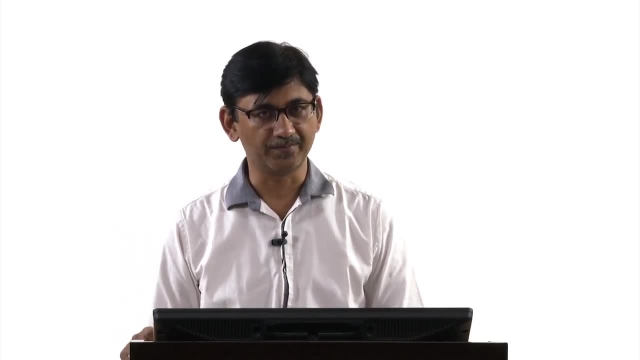 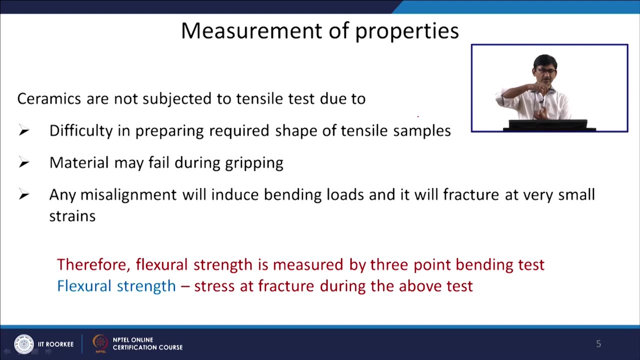 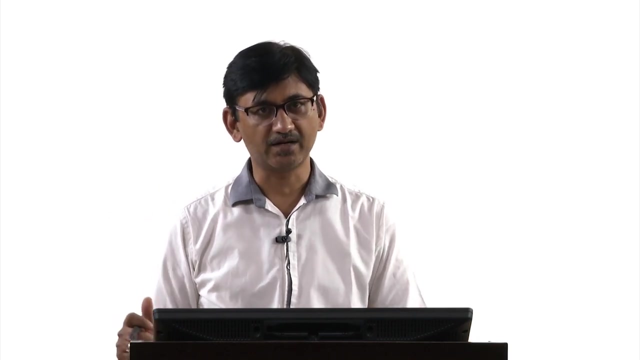 ok. So first thing is how to prepare that kind of sample. The other, very important one is because, for doing the tensile test, ok, we have seen that you have to grip the material, ok, and then you have to extend the material. So, since these are very brittle material, while gripping, 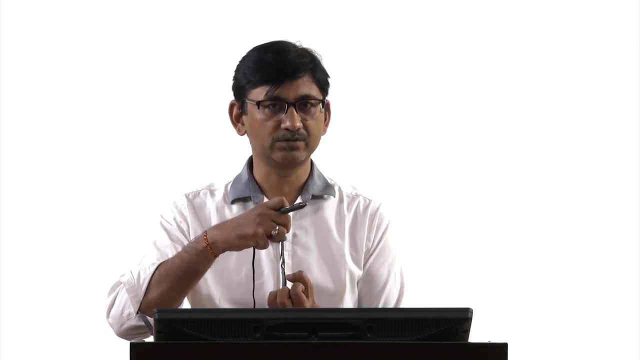 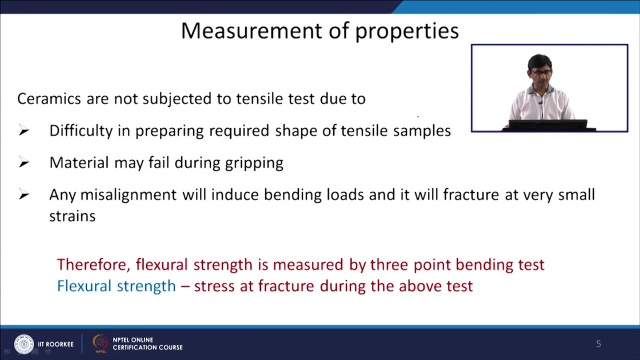 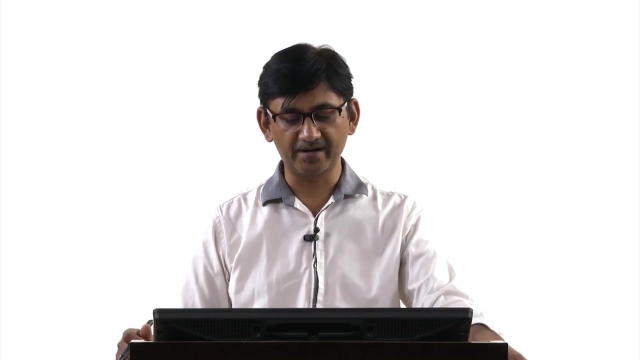 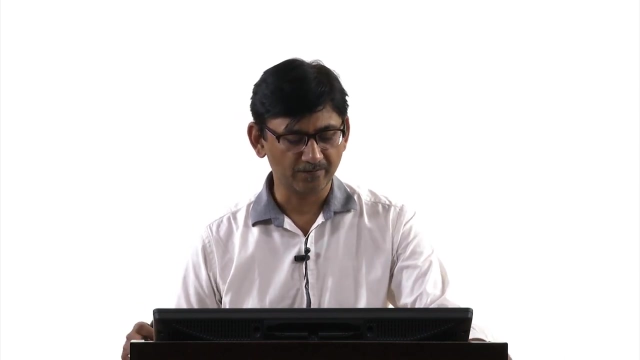 The, The stresses which will be imposed on the ceramics, that will be enough to break the material into pieces. ok, So that is not possible. And during the test, if any misalignment is there, ok, that is going to impose some bending loads on the sample and it will fracture at very small strains. ok, usually 0.1 strain or 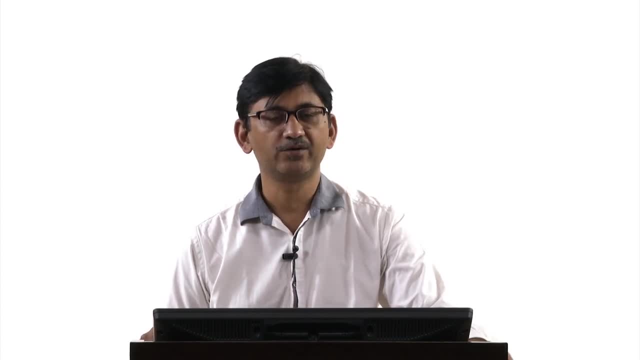 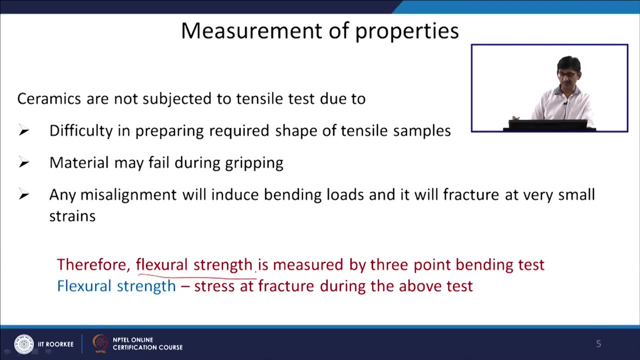 so. So that is why tensile test are not the preferred way to find out the properties of ceramics. What we measure is: the flexural strength is measured by a test called three point bending test- ok, And the flexural strength is the stress at fracture during the this type of test. three. 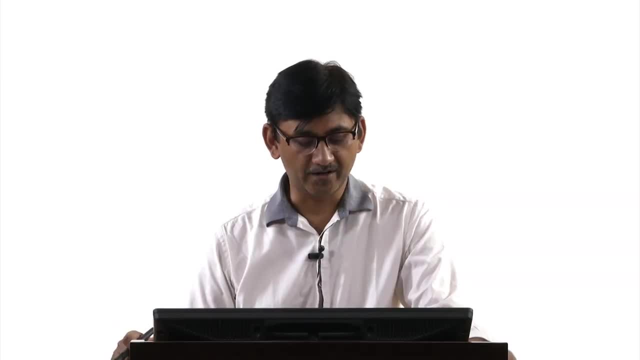 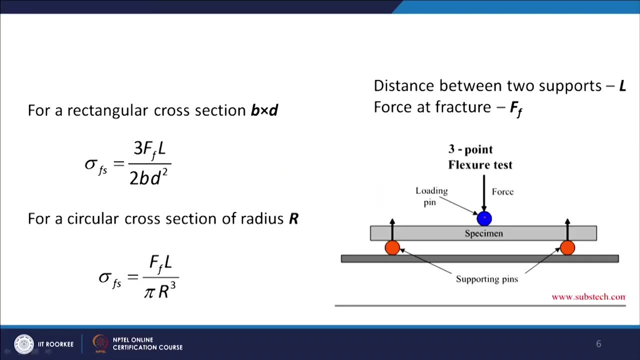 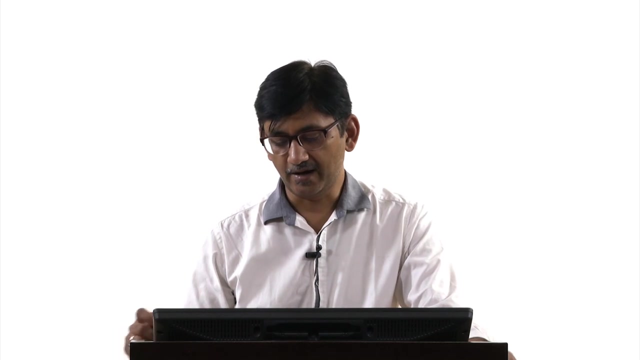 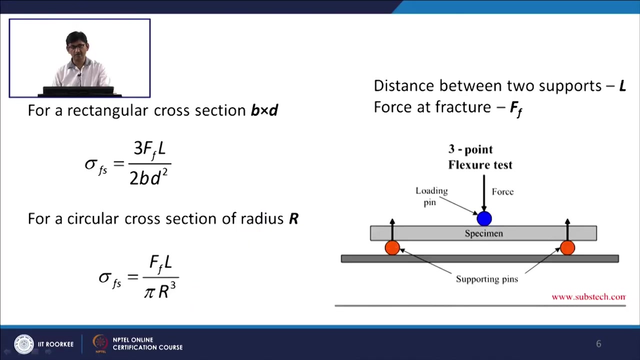 pointing three, point bending: test whatever strength you get. ok, that is what is we will be calling as flexural strength, And now I will show you that how it is done. So, basically, we can take a ceramic, simple, rock, Simple rod like this and we can simply support it on the two supporting pins here. ok, 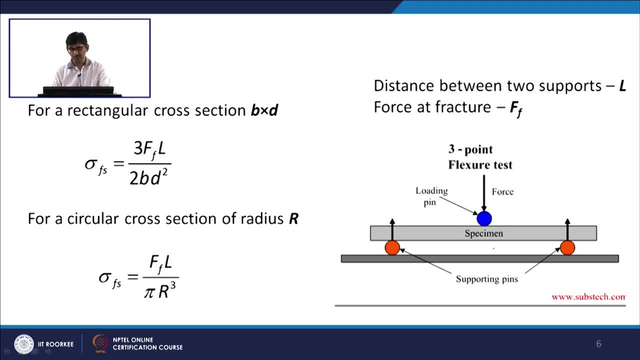 And at the centre we can apply a force F. ok, And this type of test are called three point bending test, because you are supporting the material at two points and at the third point, in the middle, we are applying the stress. ok, So what will happen? 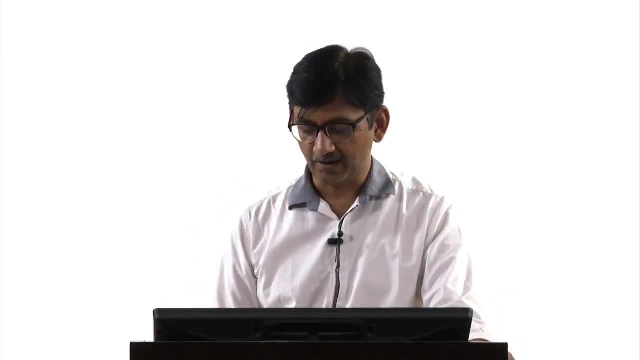 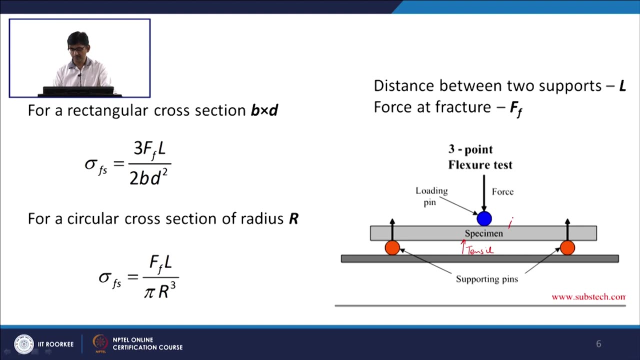 The material will bend under the load- ok. And if you are applying the force from the top, you will have tensile stresses here- ok, and you will have compressive stresses here- ok. So when it fractures, the crack will propagate from. some will initiate and start propagating. 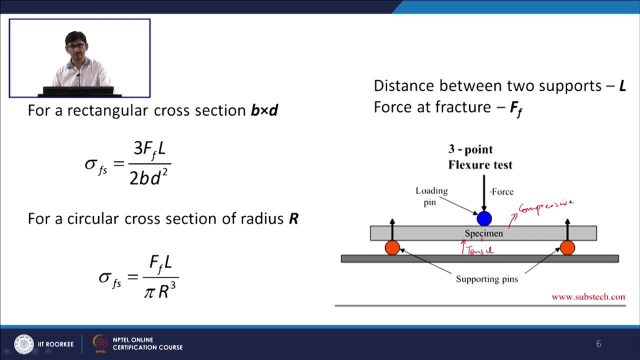 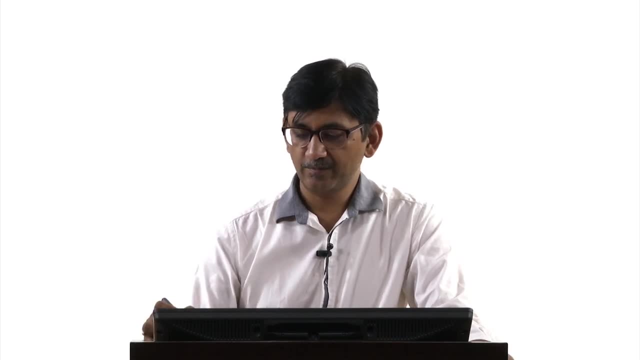 from somewhere here and then it will go through the throughout the sample and we can measure that at what force. ok, This happened. ok, and that can be used to calculate the stress it can take. ok, So the distance between the two supporting point is the we can say is L The force which? 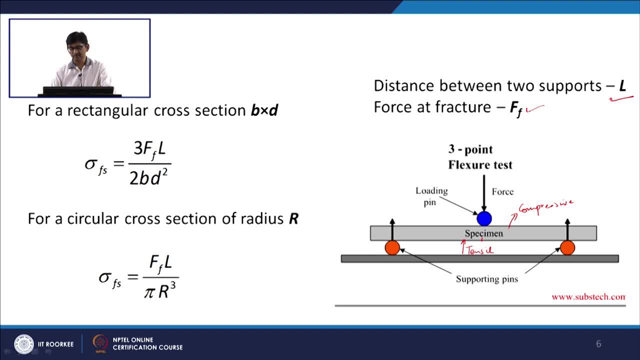 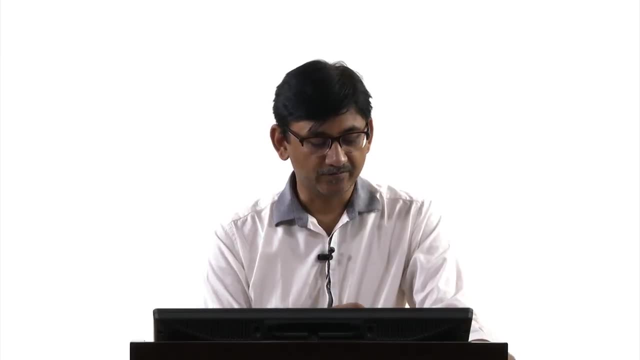 we measured using the load cell at fracture. is F sub F For a rectangular cross section ok. having a dimension of B by D, ok. so B is thickness and D is width. Then the equation for the fractural strength or the stress at fracture, sigma Fs will be: 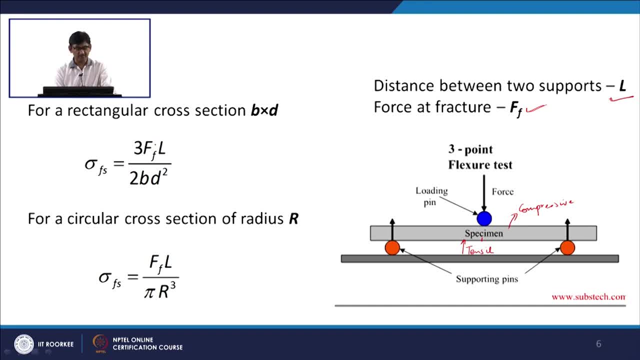 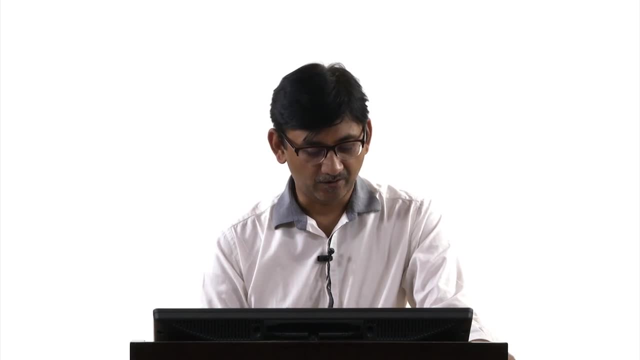 given by an expression like this, where Ff is your force at fracture, L is the length between the two supporting points and B and D are the cross sectional dimension of the material For a circular cross section of radius R. ok, the expression will be slightly different. 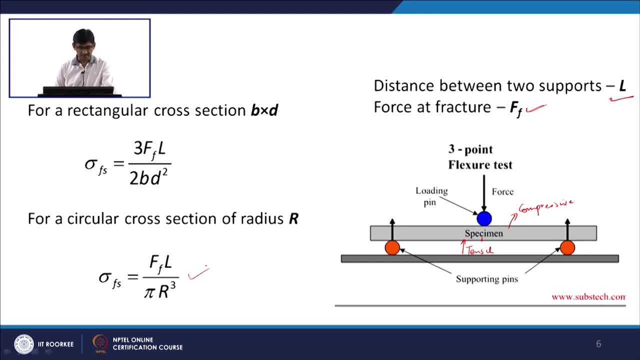 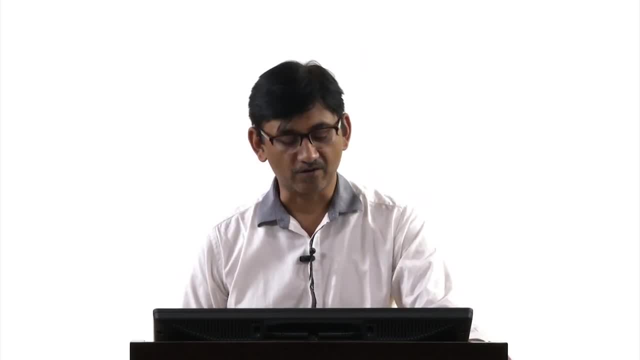 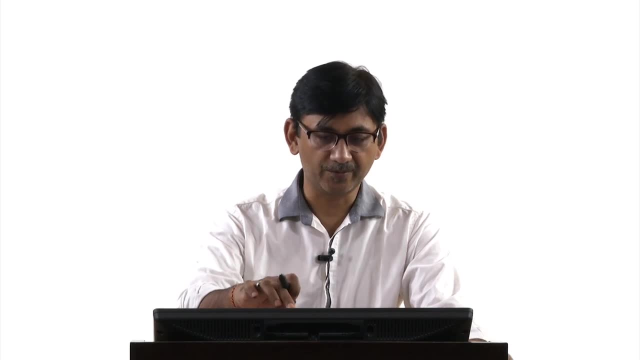 ok, It will be given by the expression given in the second case. ok, So using these values, ok, we will be able to calculate that. what is the fracture strength of the material- ceramic material? So this is what we are going to report in case of ceramics. 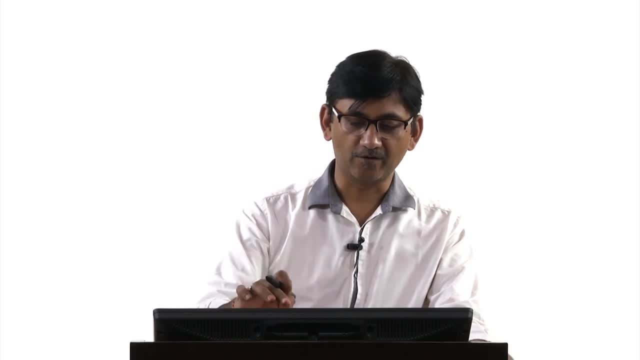 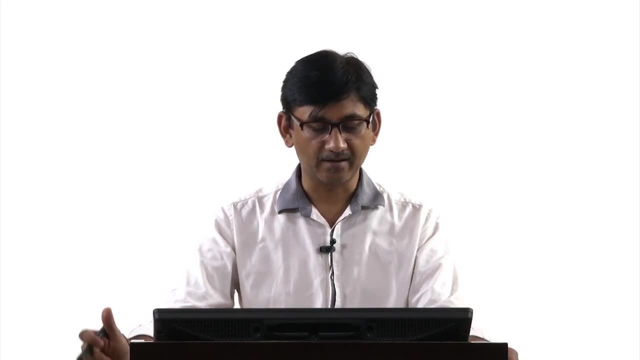 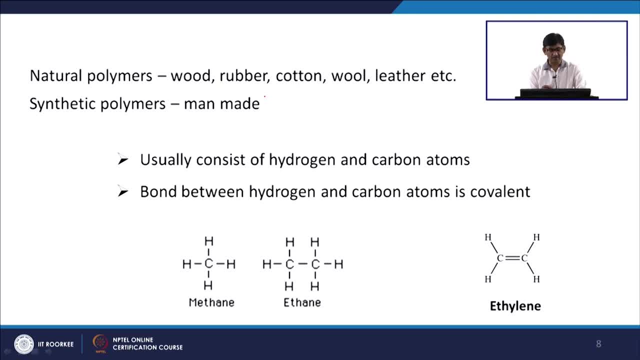 Yes, Yes. Yes, This is one of the polymer. ok, rubber is another polymer, cotton wool leather. So these are all natural polymers available to the main kind. ok. Then there are synthetic polymers which are made by man for their use. ok. 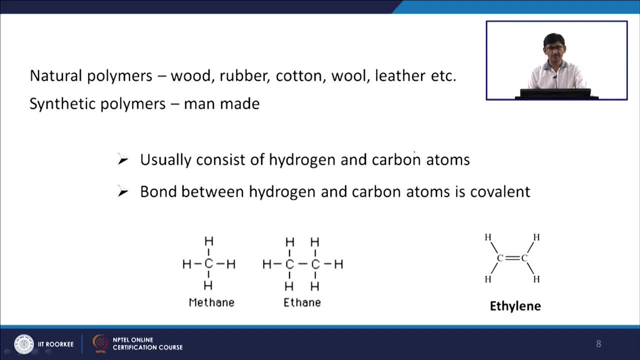 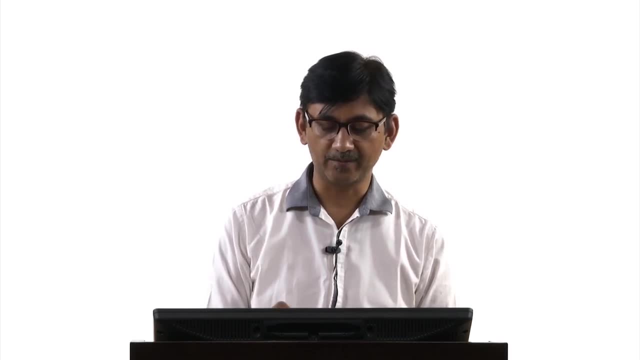 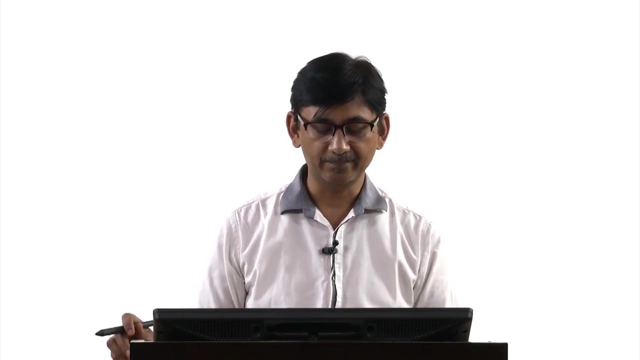 And this polymer actually consists of hydrogen and carbon atom. usually there are some other elements also or some other atoms also can be added in the molecule, ok, But usually they most of the polymer. the main component will be hydrogen and carbon atoms and the bond between the hydrogen and carbon atom will be covalent type. 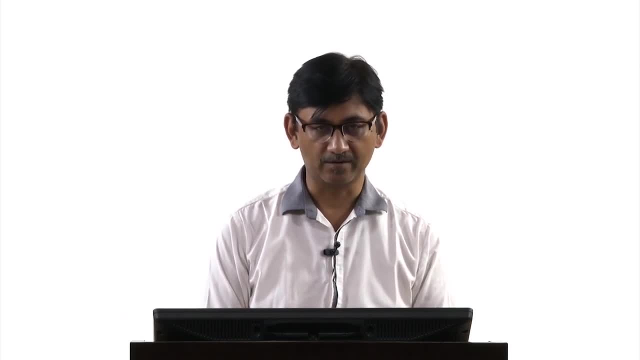 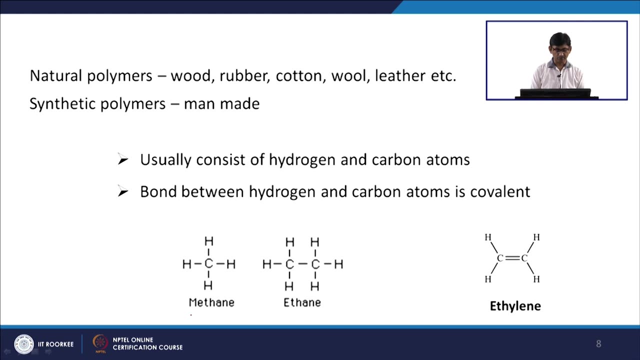 So it will be like this: carbon atom is sharing. each carbon atom is sharing one electron with each of the hydrogen atom to so that they have a stable configuration. So in this case it is methane when it is sharing with 4 hydrogen atoms. ok, 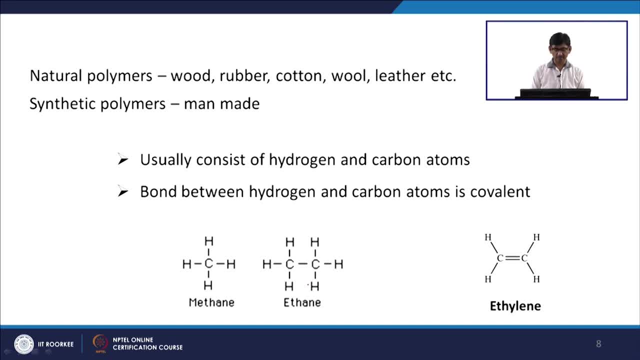 If you combine 2 carbon atoms and remaining are shared by the other hydrogen atom, then it is ethane. ok, If we do not have the 6 hydrogen atom, then there has to be a double bond between the 2 carbon atoms. ok, In that case it is called ethylene, ok. 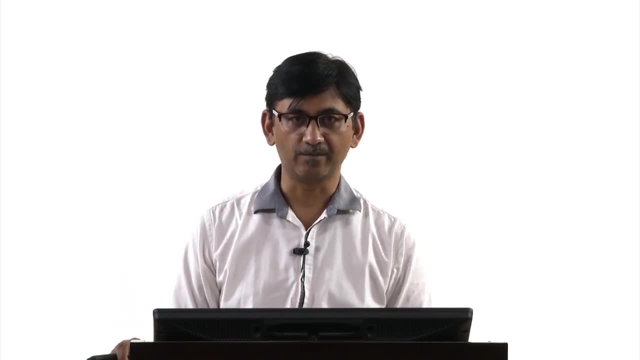 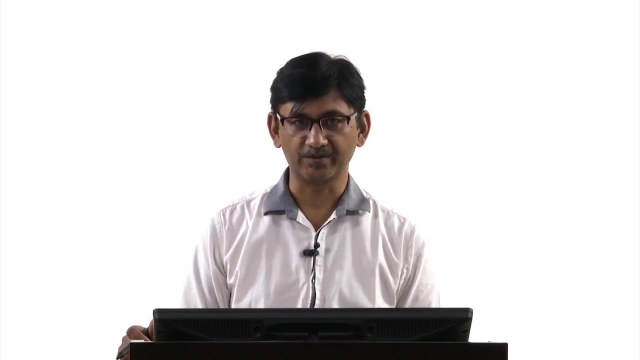 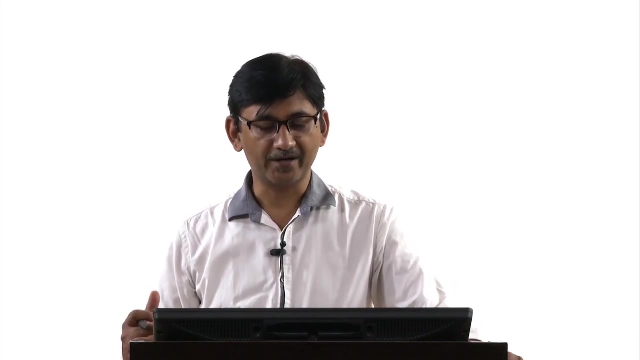 So you can have different types of molecules Which can be used to make a polymer by having different type of bonds between the carbon and hydrogen atoms. So if you see the molecule of a polymer, these are called macromolecules. ok, Because they are very long chained molecules. ok. 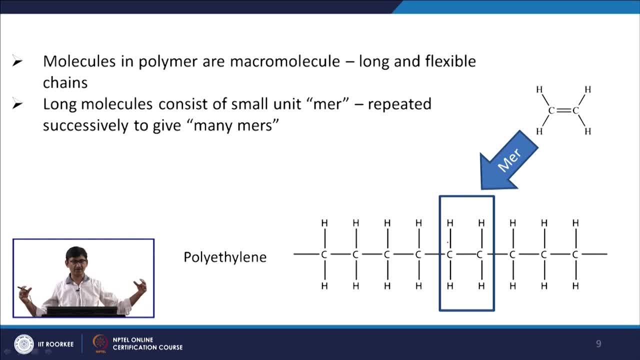 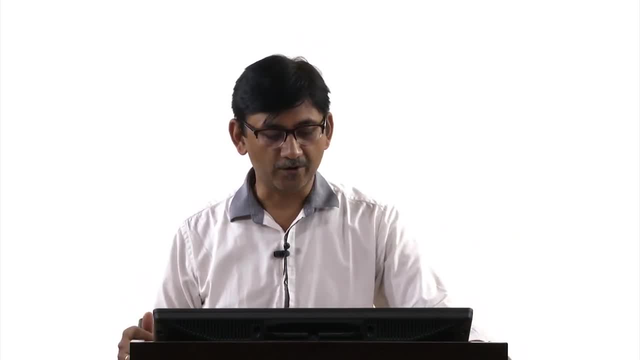 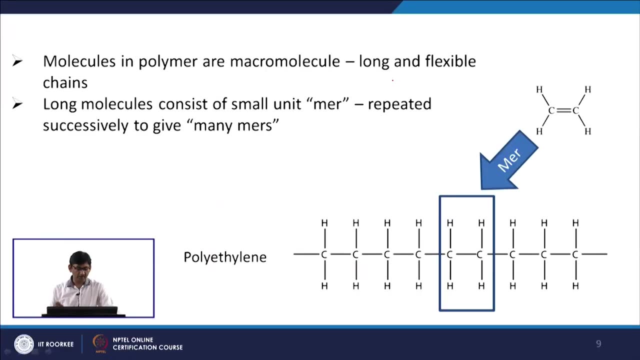 So one molecule may consist of very large number of atoms and it may be in like a chain form- ok. So molecules in polymer are macromolecules, which are basically long and flexible chains. ok, And this long molecules consist of a small unit called mer. ok, 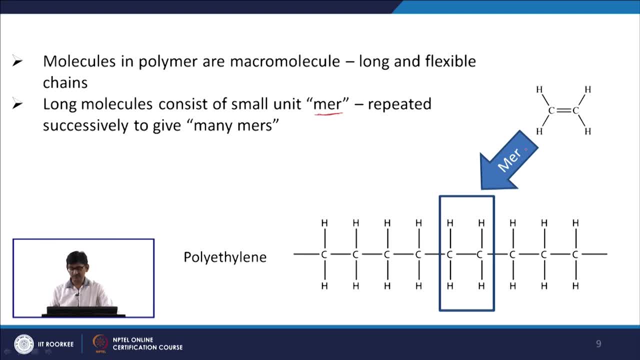 So one small unit can be shown here, ok, which is basically ethylene molecule. So this is the mer, the 2 carbon atoms and 2 hydrogen atom attached to each carbon atom. ok, So this is one single unit which can be repeated. 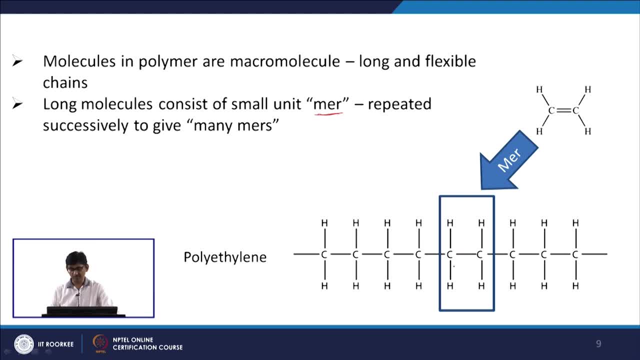 Ok, So one unit is shown here. ok, This can be now repeated again and again. ok, to make a big chain of these small molecules. ok, and make a big molecule. So these are repeated successively to give many mers: ok, and that is why these are called. 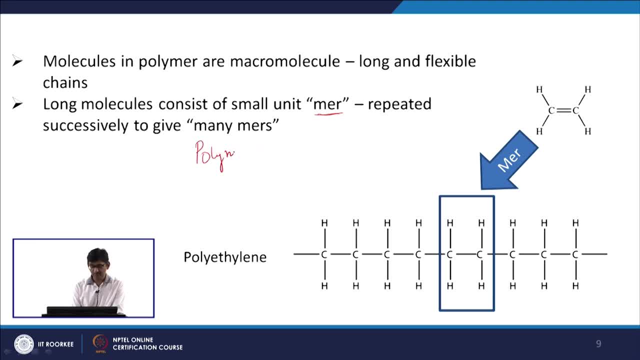 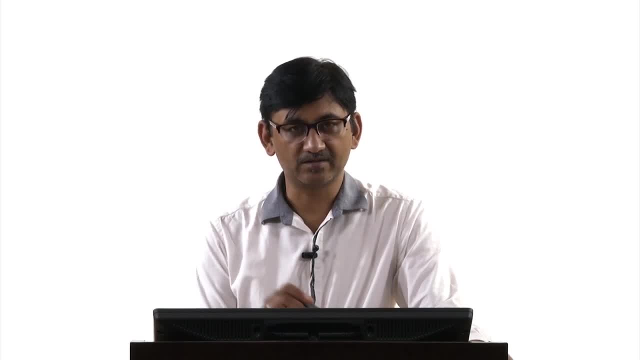 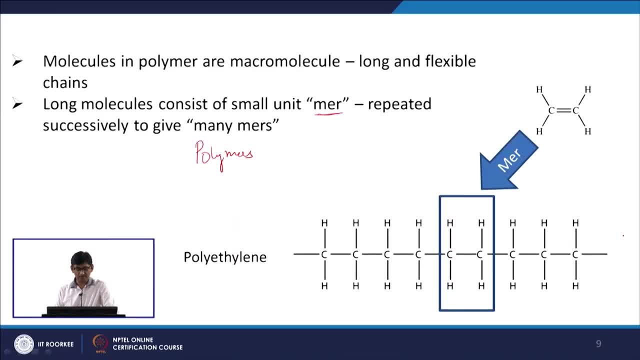 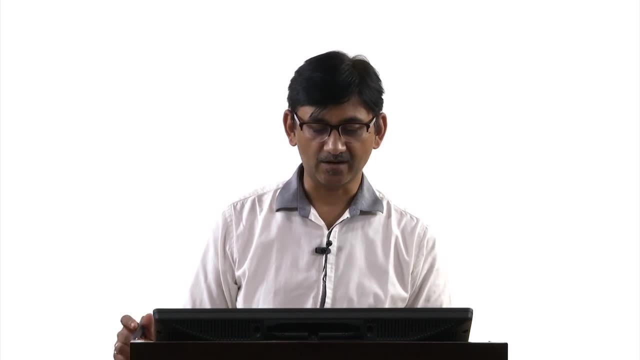 So this is a very popular polymer, polyethylene. ok, So one ethylene can be combined together to create a long chain of molecule, The chain shape and structure, if you want to see. ok, Chains are not straight, but in zigzag shape. ok, 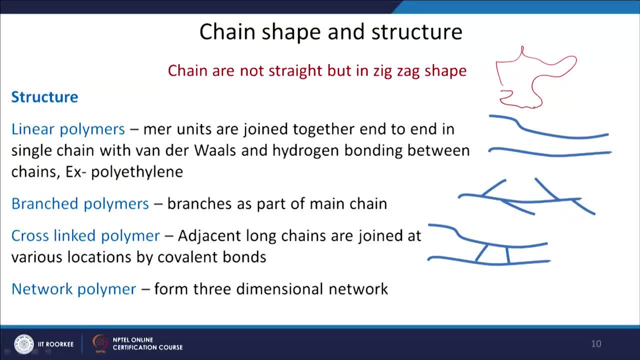 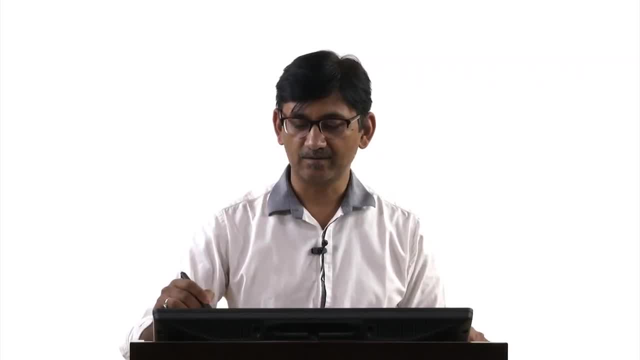 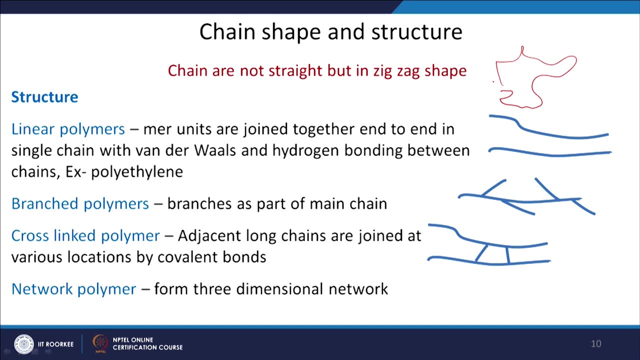 So chain can be like this, also may be something like this: ok, okay, very long chain, and basically all these small molecules keep attaching to each other and you can make a very long chain like that. okay, so these are not straight chains, but 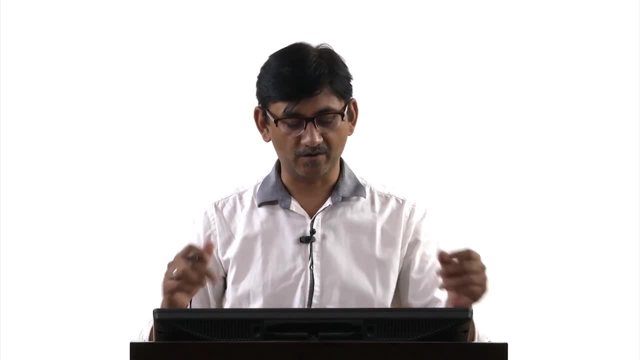 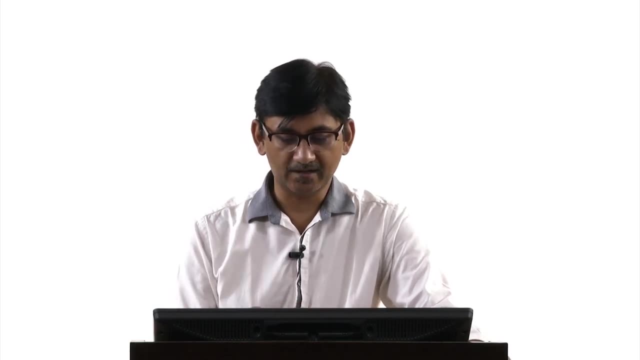 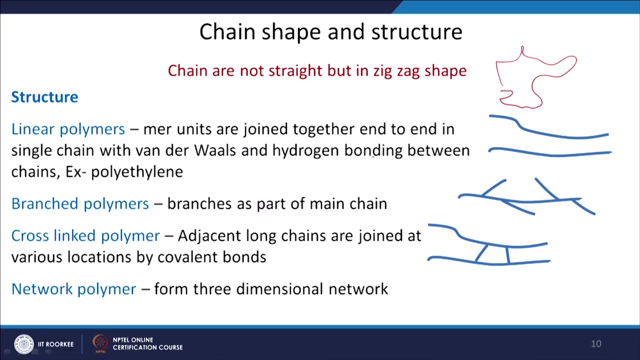 maybe arrange in a very zigzag fashion in the overall structure so we can define the structure according to this. okay, so linear polymers are basically mer units are joined together end to end in single chain with wonder wall forces and hydrogen bonding between chains. example: polyethylene. okay, so basically in this case you have this: long chains, okay. 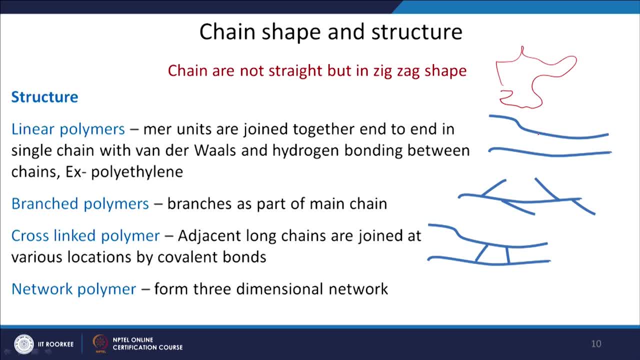 of macromolecules and there may be between the carbon atoms and the hydrogen atoms. okay, there can be some wonder wall forces can be there, okay, or hydrogen bonding can be there between the 2 big molecules, okay, so you have 2 chains and between the 2 chains there. 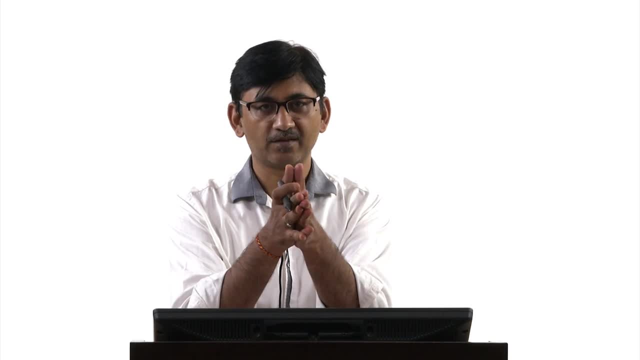 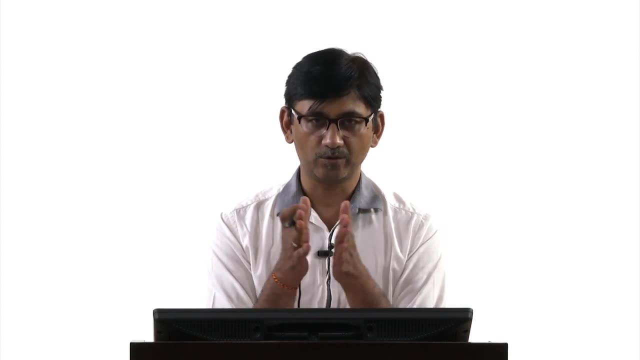 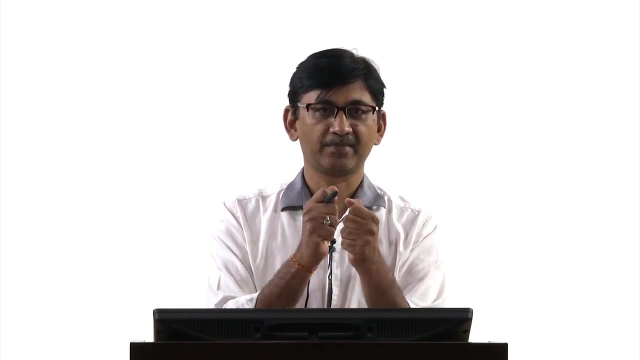 can be. some kind of forces can be there. okay, these are either wonder wall forces and or hydrogen bonding, and in both cases we know that these forces are very weak. okay, so it is not going to hold it very strongly. you can have some relative movement between the. 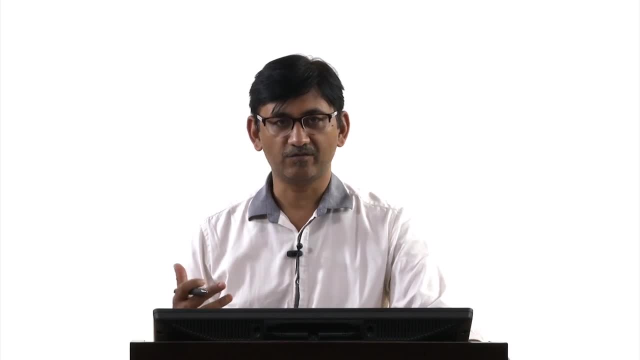 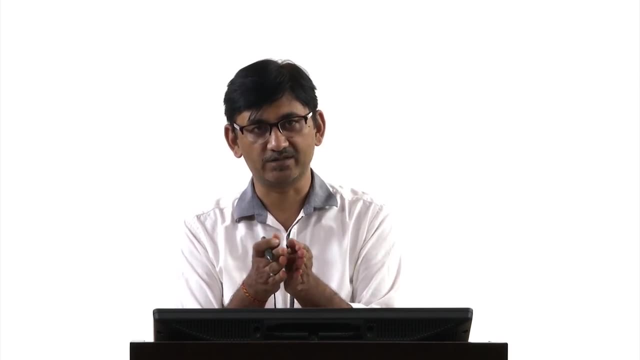 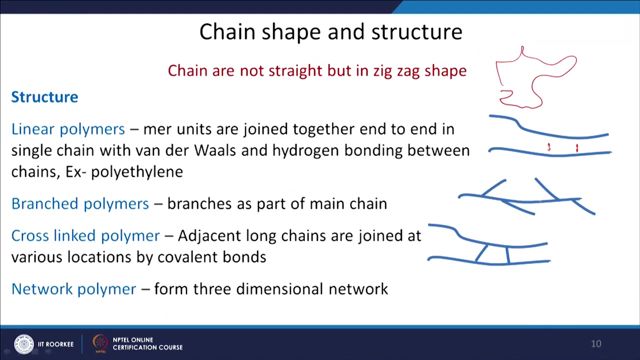 chains. So these are not very strong forces, but they can keep the molecules kind of together by having a small force acting on them. another kind of polymers can be branch polymers. okay, in this case you can have a small branches coming out of the main big chain, okay. so 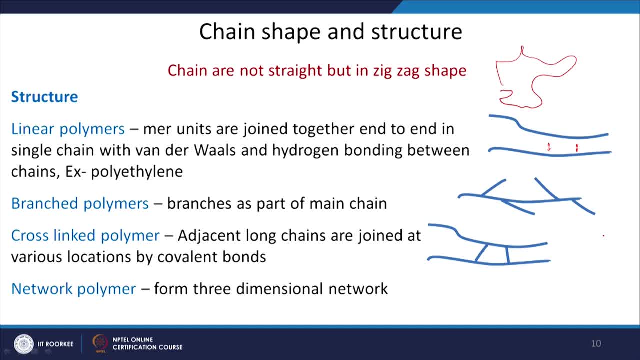 these are called branch polymers. then you can have cross link polymers. in this case now, the 2 big chains are kind of connected with each other with cross linking. okay, so these cross linkings are there. okay, so adjacent long chains are joined at various location. 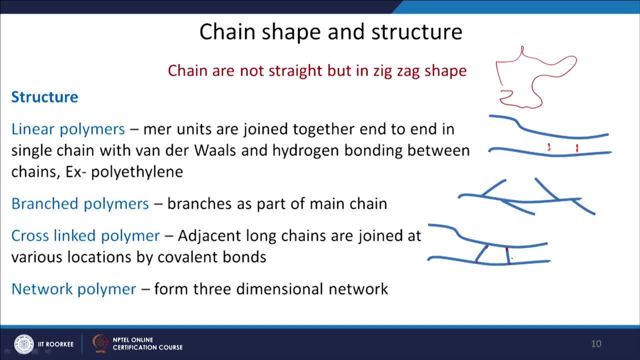 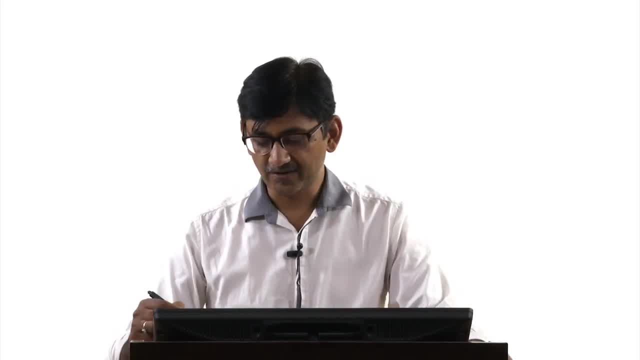 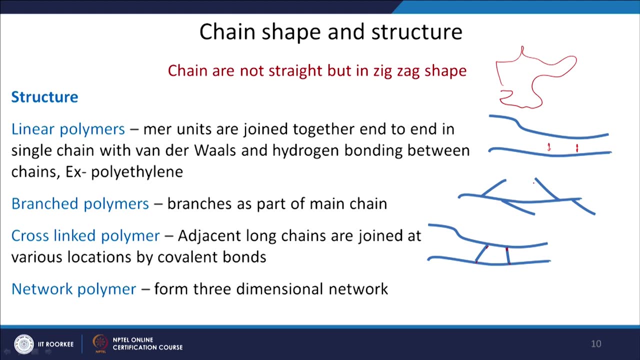 by covalent bonds. okay so, and then there can be a network polymer which forms a 3 dimensional network. okay, so you can see that, as we are going from this simple type of arrangement, okay, 2. Branch type and then to cross linking type and to network polymers. you can understand. 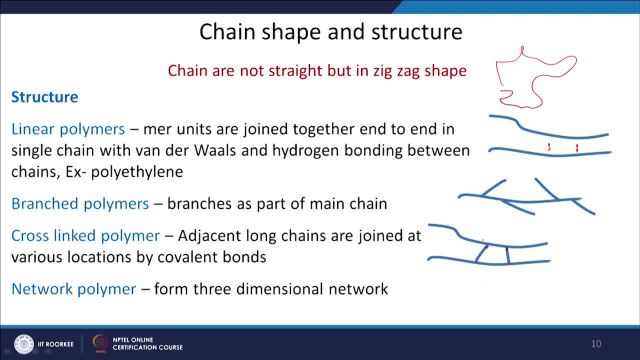 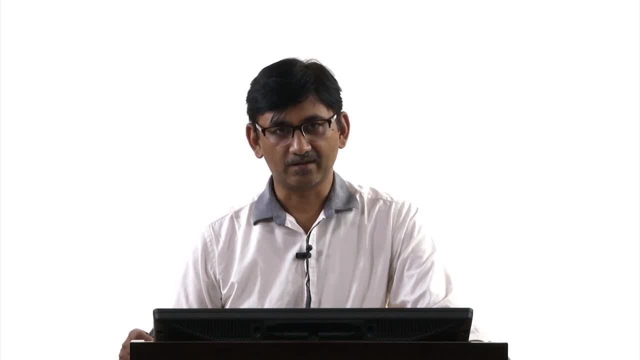 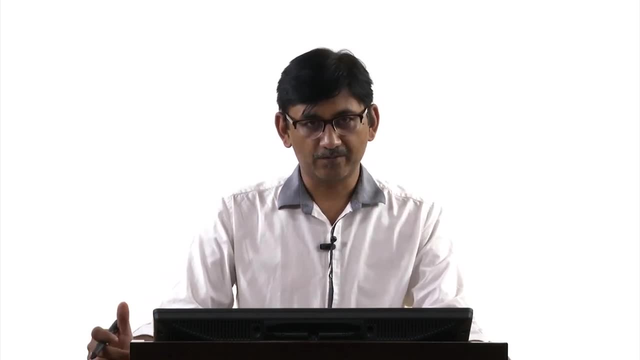 that the strength of the polymer will increase in this way. okay, because it will be more difficult for you to deform the polymeric chains. okay, during when you are applying any stress. okay Now, if you want to see in terms of crystallinity, that whether there is any crystalline nature, 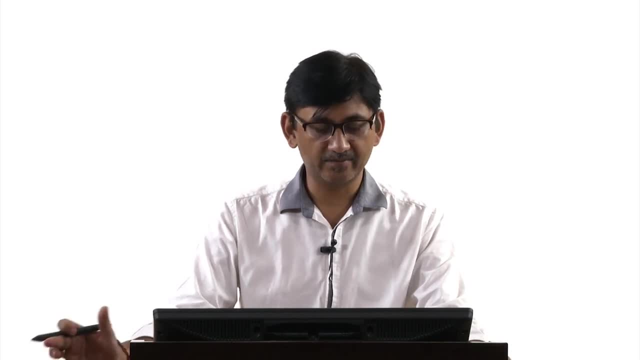 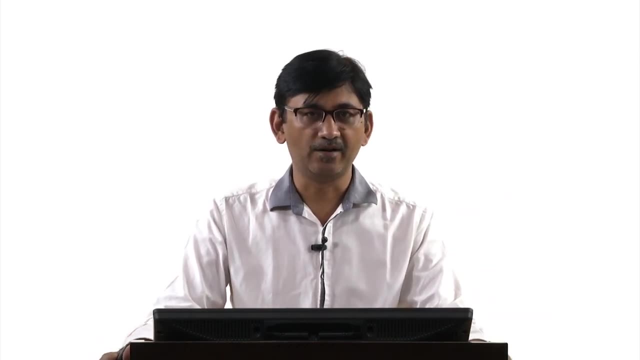 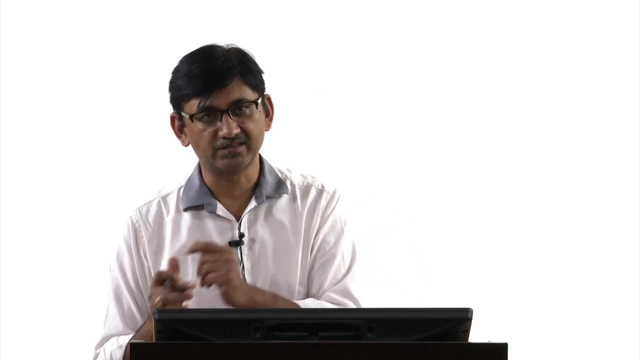 is there for polymers. 3. Polymers can be divided into 3 types. okay, an amorphous polymer means there is no long range arrangement of atoms. okay, like what we see in metals, that atoms are arranged in a very nice fashion according to their crystal structure. okay, in case of amorphous polymers. 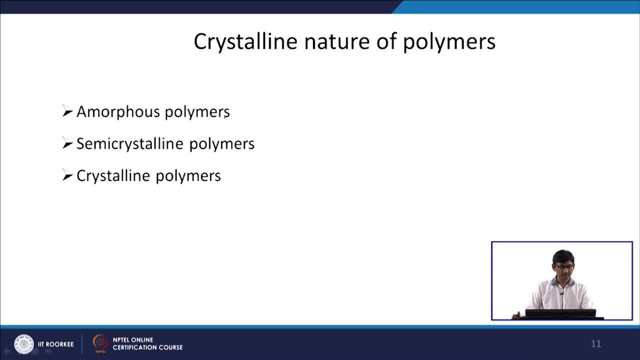 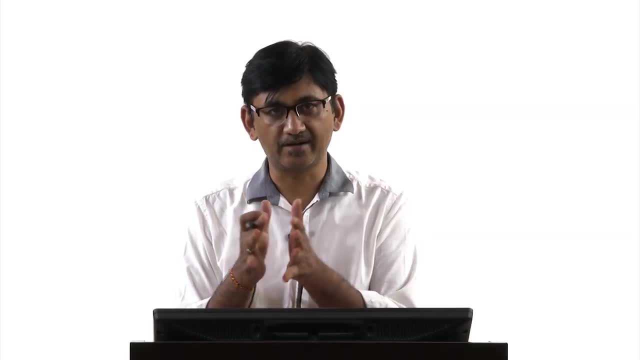 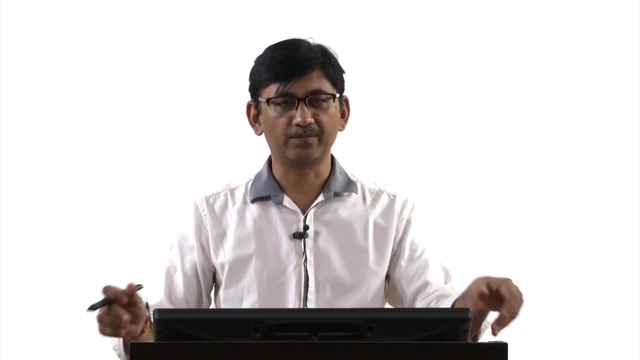 there will not be any arrangement of atoms. okay, then there can be semi crystalline or crystalline polymers. okay, In this case the atoms are arranged in a particular manner. okay, you can have a repeated arrangement of atoms and you can do some XRD analysis to find out the crystallinity in the polymers. 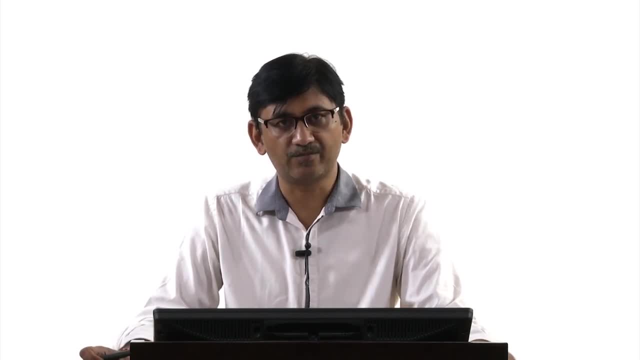 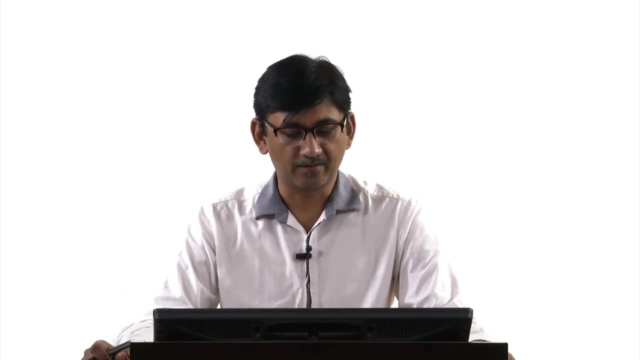 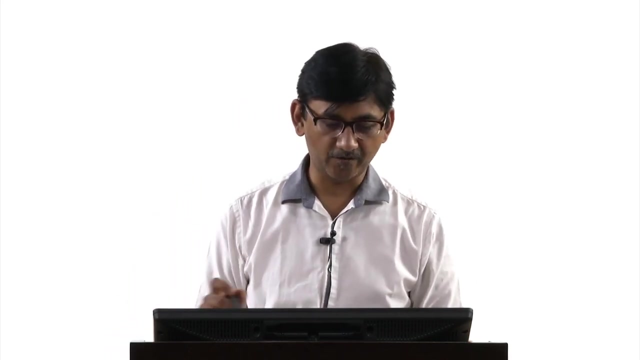 so it is possible to have a crystalline nature of polymer. that means there will be some repeated arrangement of atoms in the polymer, okay? 4. Stress strain curves. Now coming to stress strain curves, Okay, of polymers. okay, the elastic deformation due to elongation of chain molecules by bond. 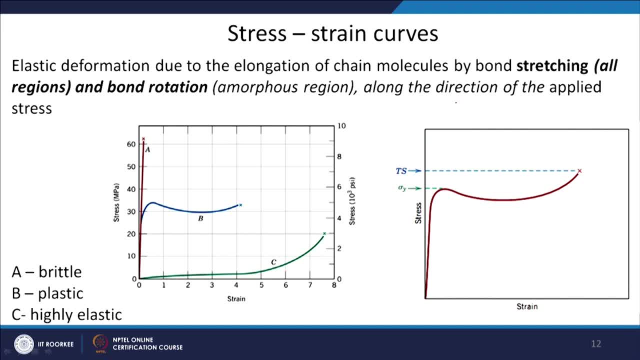 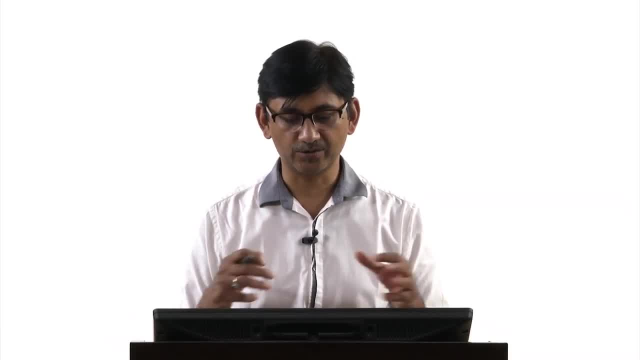 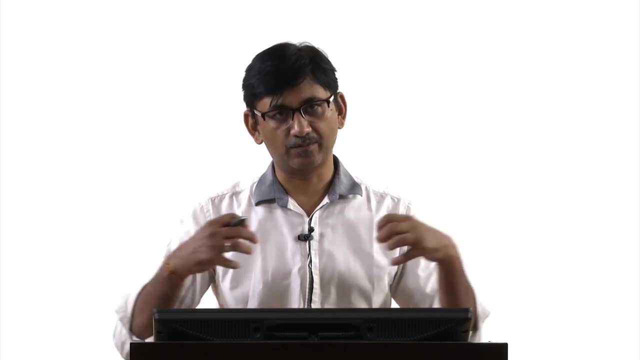 stretching and bond rotation along the direction of the applied stress. so the elastic deformation part, if you see in the polymers, okay, it is due to the bond stretching and bond rotation along the direction of the applied stress. So in this case also the bond stretching will be there between the 2 atoms. okay, then there. 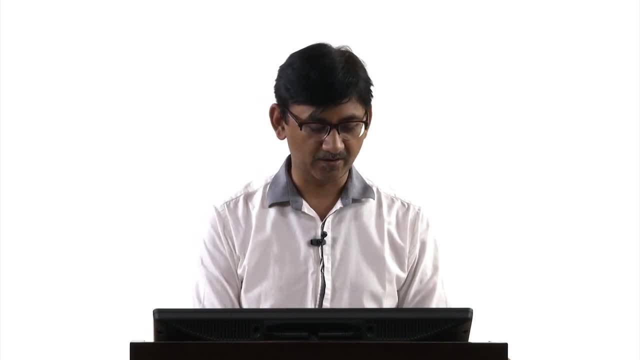 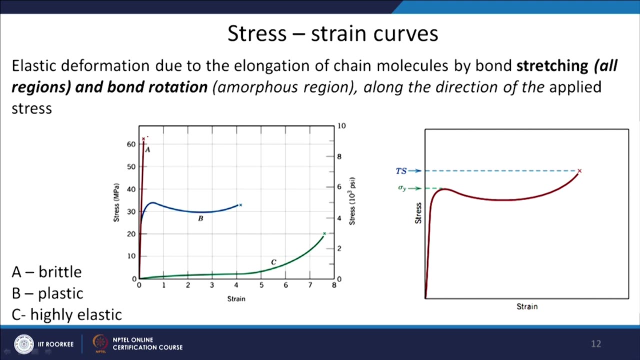 can be 3 types of polymers. The polymers are shown here. okay, the polymer A is a brittle polymer, okay, so you can see that only the elastic part is there and then the fracture took place. then there can be a plastic one which will, which is shown here also. so this is the B type here. so it shows. 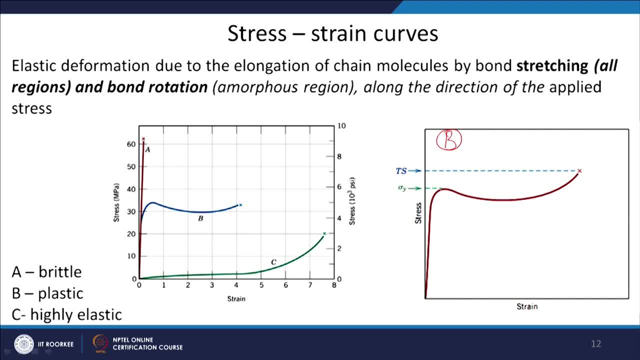 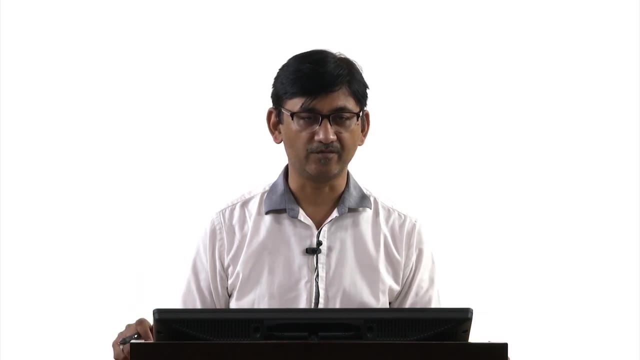 the elastic part here. okay, then you have the yielding of the polymer and then you have the Plastic deformation and the maximum stress at which the polymer will fracture. okay, so this is a typical polymeric stress strain curve for a polymer which shows plastic deformation. 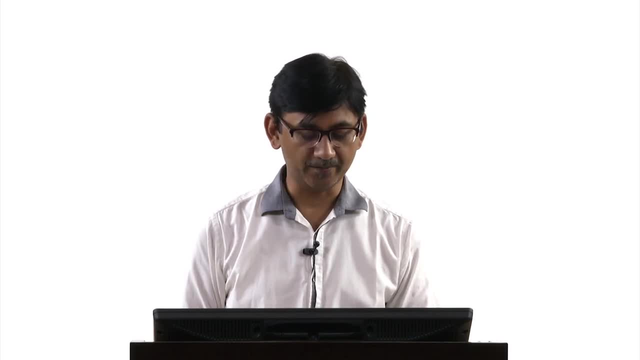 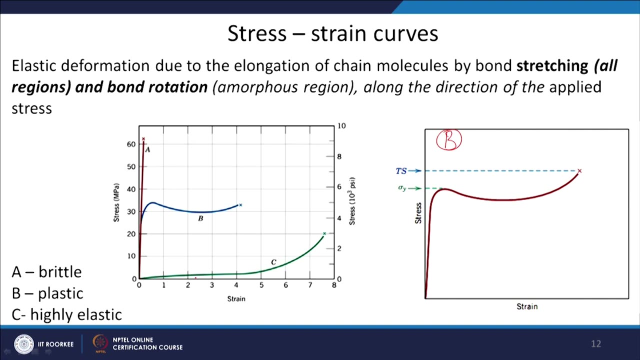 Then for one which is shows very highly elastic deformation. okay, you will not see this yield stress. and then the plastic part, but it will start deforming and you can see that the young's, the modulus is very small for this kind of polymers. okay, so it start deforming, so very 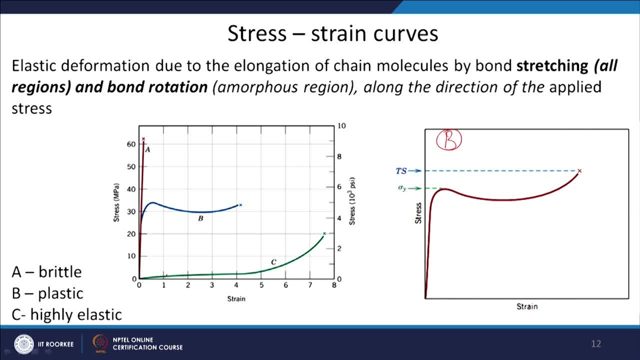 high strain is there without any corresponding increase in the stress. okay, and when the all the chains are kind of stretched, then you start seeing some deformation. okay, in the plastic. it also may not be plastic here. it will be still in the elastic range and 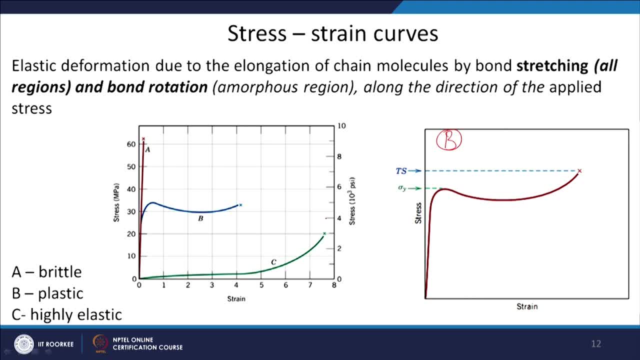 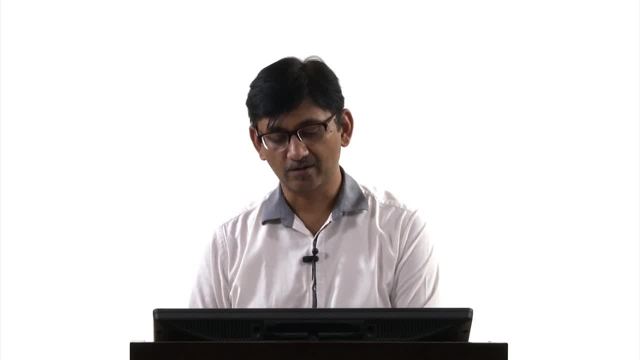 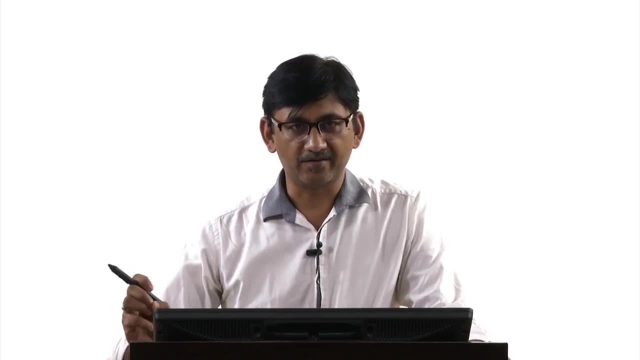 then it will fracture at this point. Okay, So this is how the typical stress strain curves will be there for different types of polymers. Now we will come to the composite materials. so we are not dealing in lot of details of these mechanical properties of these materials, just trying to get introduce you to different. 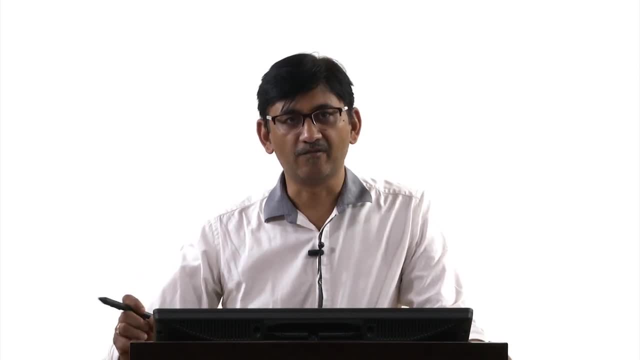 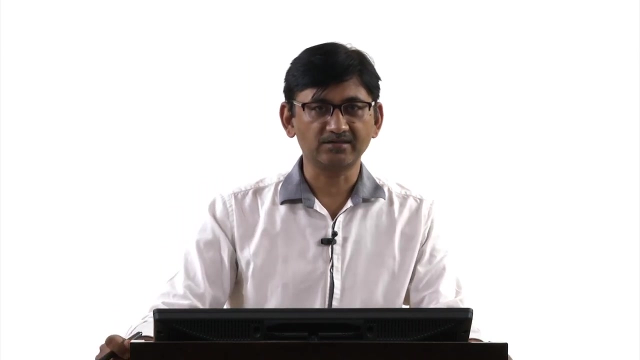 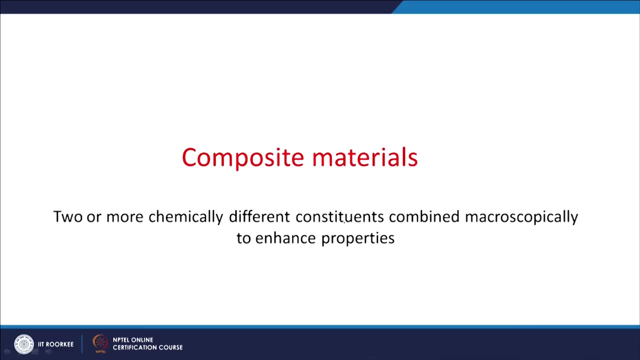 types of material, that, what, how they behave, what is their structure, and they have, of course, in engineering application also. they have usage now in different components. Then there can be another class of material which is called composite materials. so in this basically you have two or more chemically different constituents combined macroscopically. 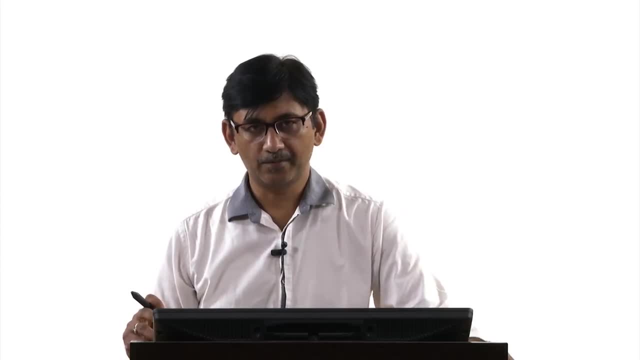 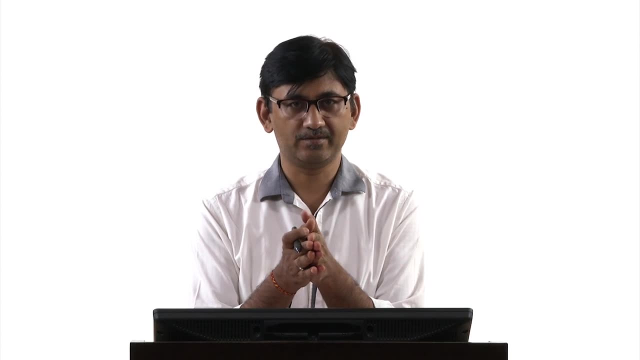 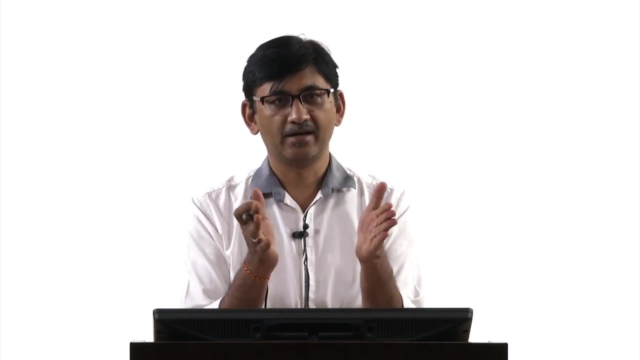 to enhance properties. So in this case we add or we combine two different material which are chemically very different to each other, and these are macroscopically combined in a way that they you can easily see that where the one constituent is there, where the other constituent is there, 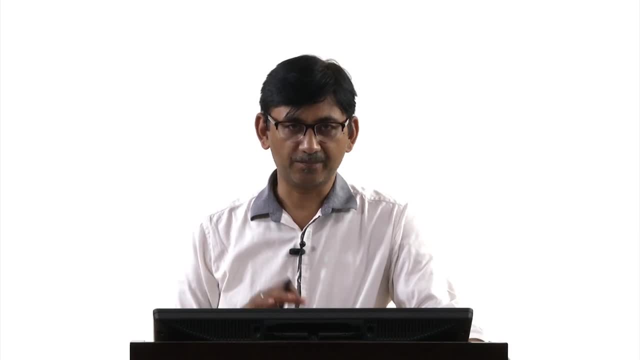 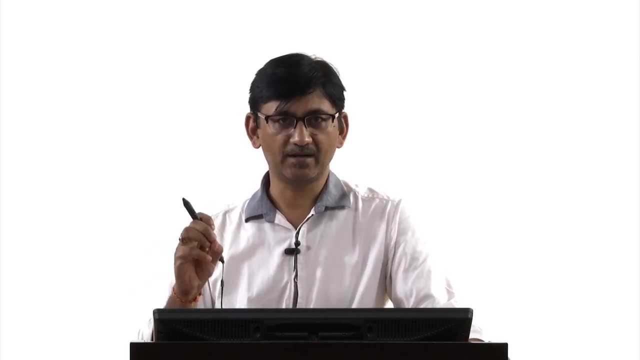 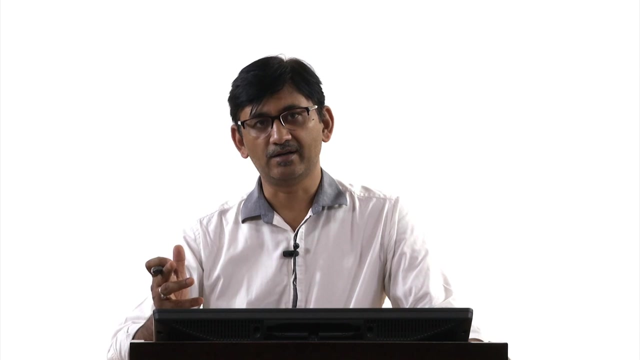 So in the sense it is not. you cannot compare this with this. Whereas with the alloys, where you have precipitates or maybe some other phase, those are microscopically, at the microscopic level. you have in situ reactions to make those alloys, whereas in 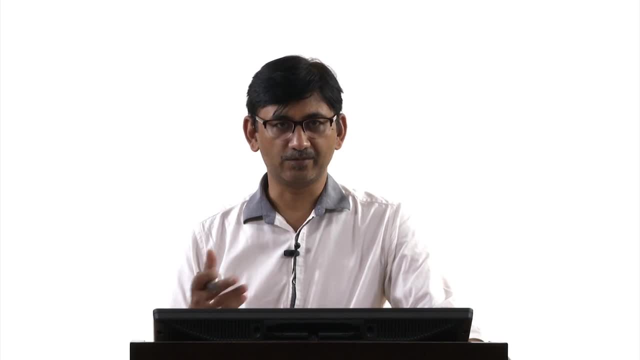 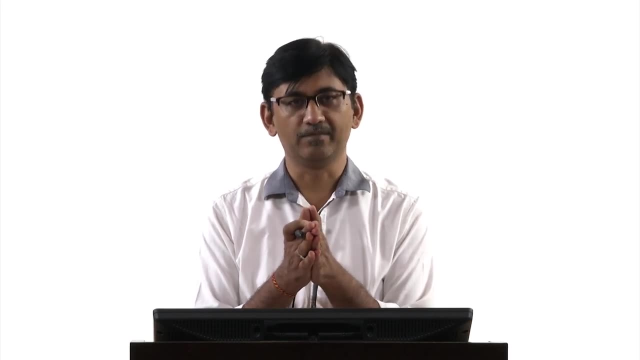 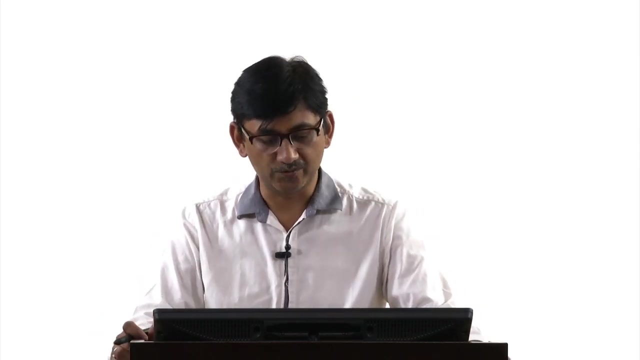 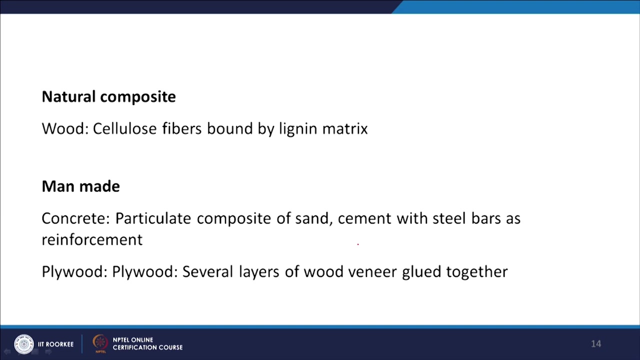 composites. there are no in situ reaction. we kind of add two different constituents- macroscopically means you can, which you can easily manipulate, And then you make a composite of two different constituents. Some of the example- natural composites, if you want to see one- is wood which contains 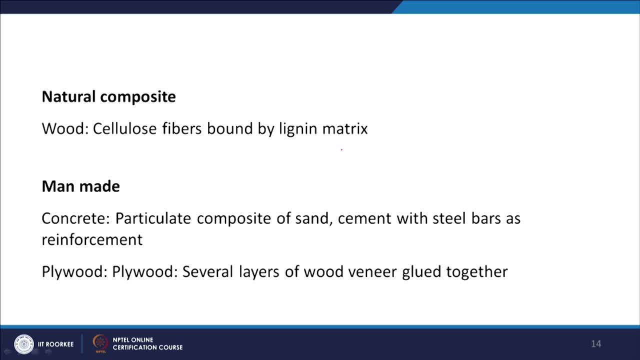 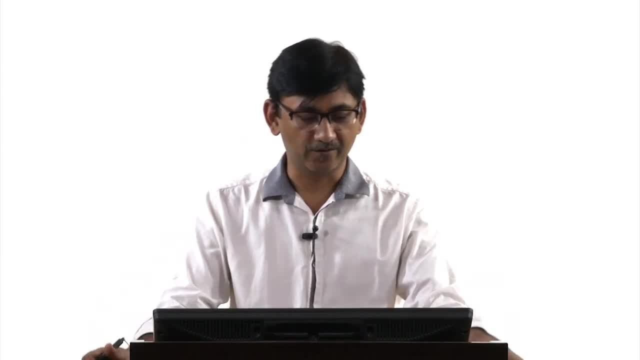 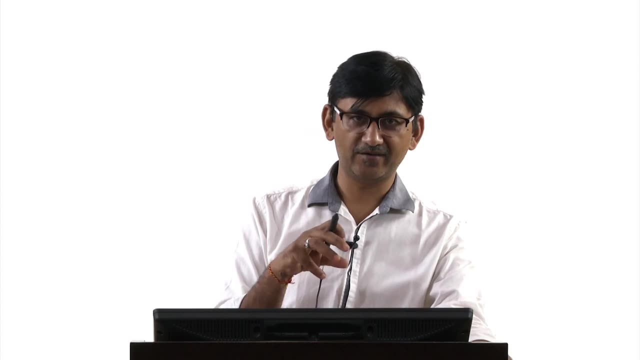 the cellulose fibres bounded by lignin matrix. So you have two different constituents and they are coming together to make wood. Main made concrete can be a very good example to understand. So you have a particulate composite of sand and cement. 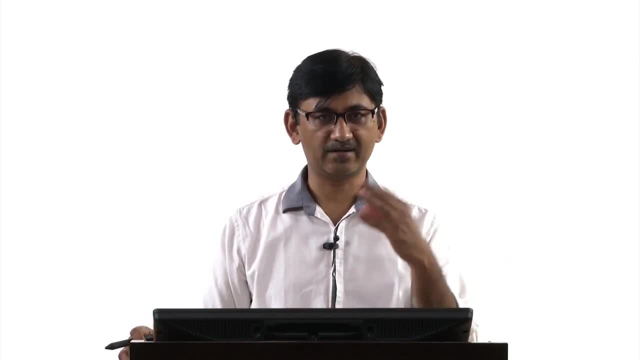 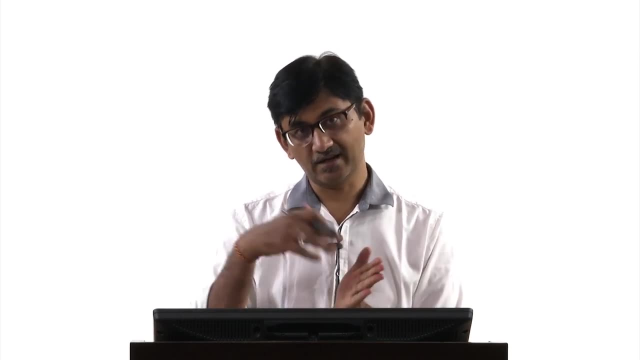 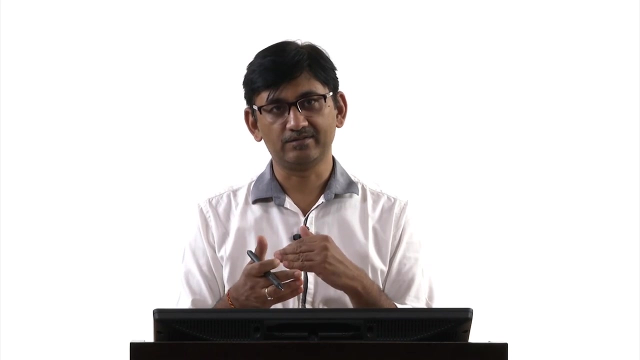 We are mixing them together. Cement is a separate constituent, sand is a separate constituent, So it can be a particulate composite- The other way of looking at it, as when you make any column or beam, you add this mixture of cement and sand. 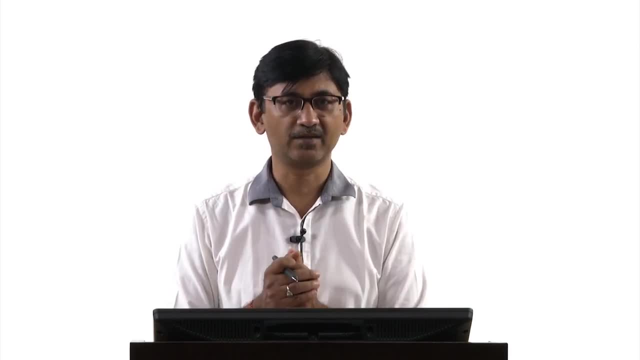 And you also have reinforcement in form of the steel O 1. 책 is now a composite of calcite. 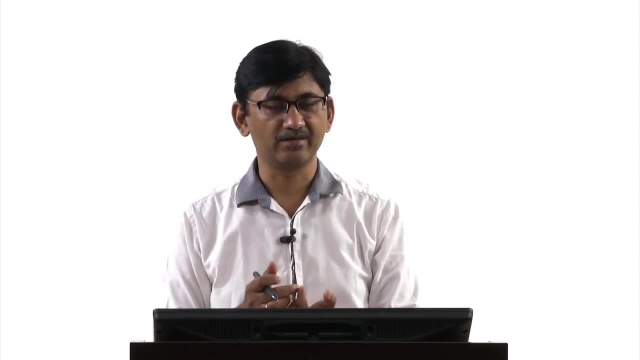 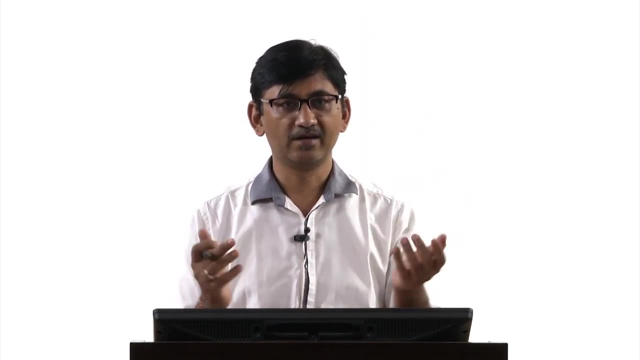 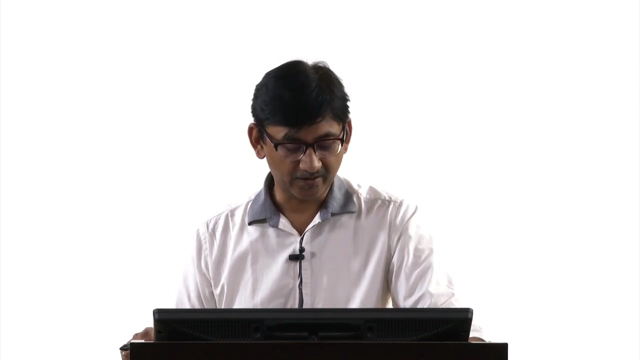 of kind of a fibre composite can be. you can look at, look at like as a fibre composite that a steel bar is there and around that you have cement and sand mixture. okay, Apply wood is a very good example of composite. okay, several layer of wood veneer is glued. 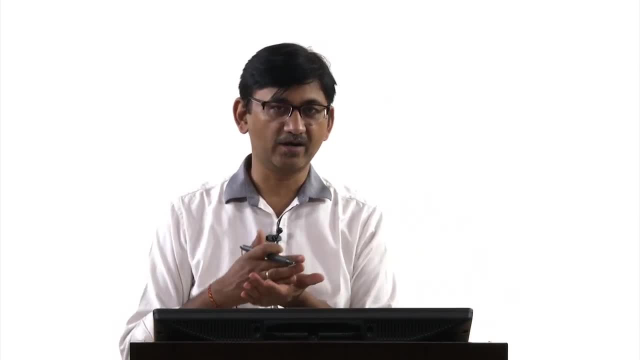 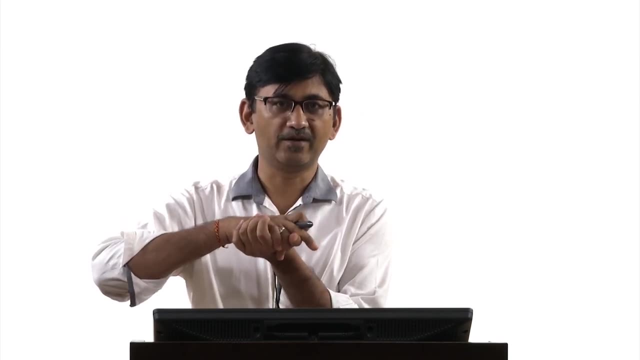 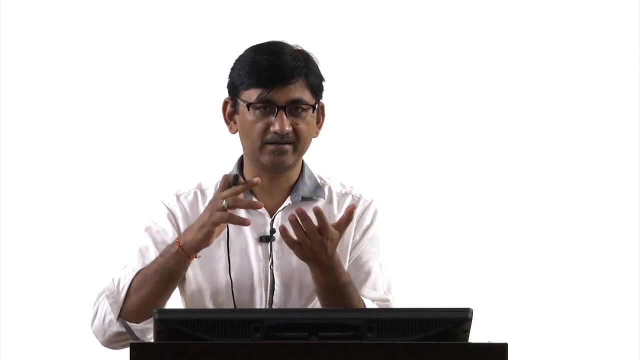 together. So, if you see, apply wood, if you cut it, you will see there are individual layers of wood, okay, which is pasted together, okay. So by making a composite like this, you can increase the strength of the wood and it these: 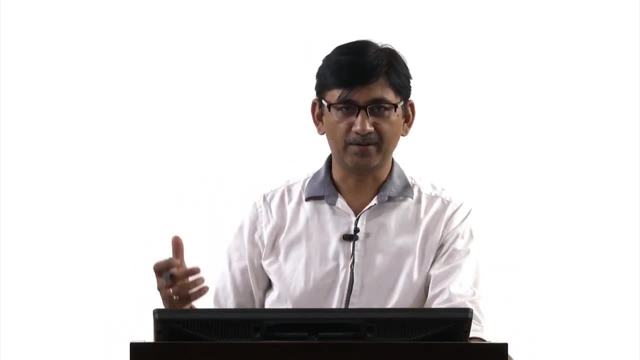 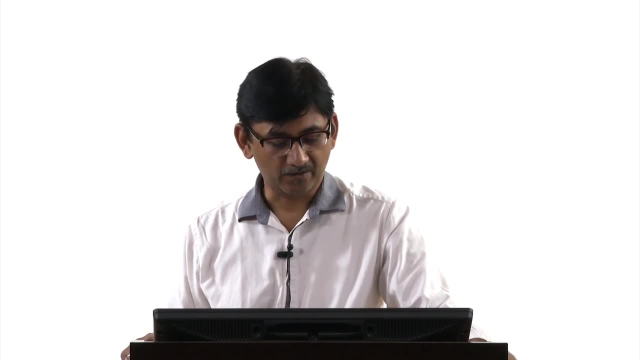 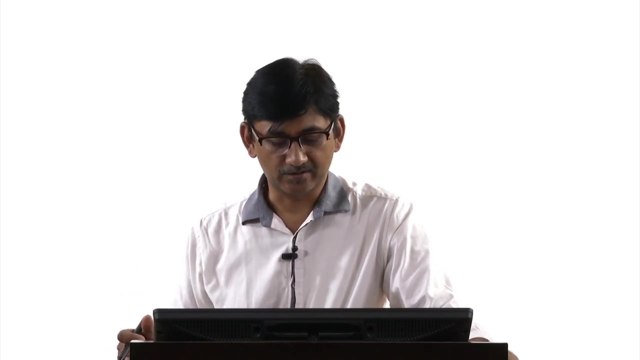 are very high strength material. okay, and that is why they are used in a lot of different application, as a structural material also okay, So apply. wood is a very good example of composite. similarly, the RCC, the reinforced concrete, is a very good example. 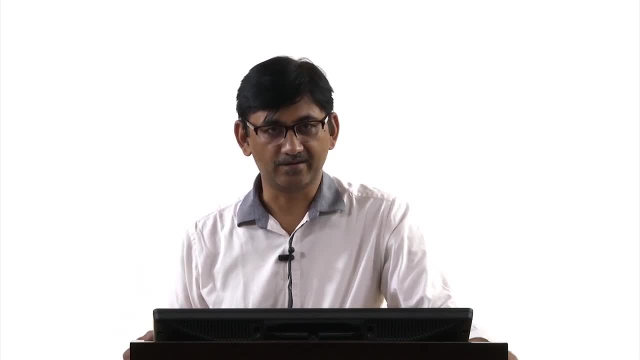 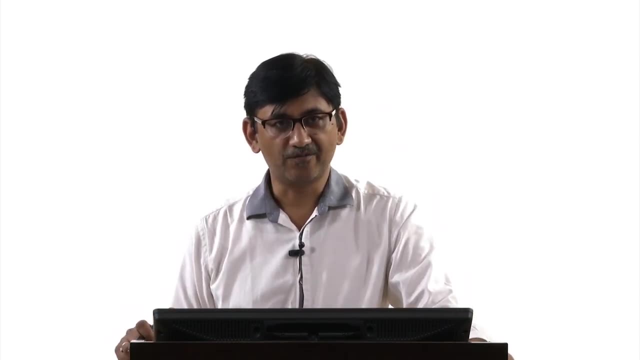 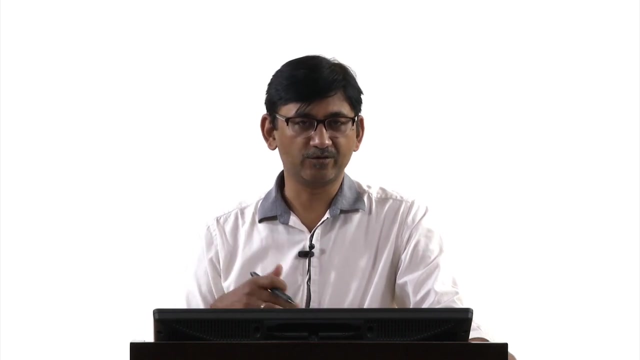 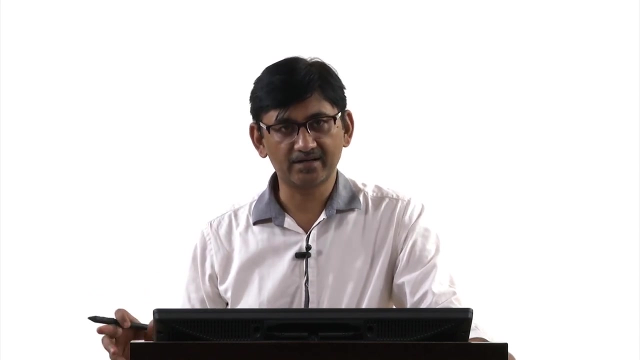 Okay, of composite. that how the composite materials can be made. So primarily composite consist of matrix. okay, as you can see in terms of wood, that apply wood which we were discussing, or the concrete which we were discussing. okay, So it will contain a matrix and then it will contain a reinforcement. okay, 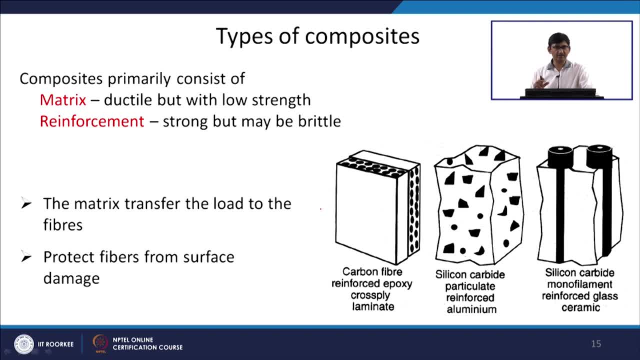 So the matrix is. So the matrix is usually: if you take metals or polymers, okay, it will be ductile. okay, but has low strength, okay. So problem with the matrix is that, though, it is a ductile but it has low strength. 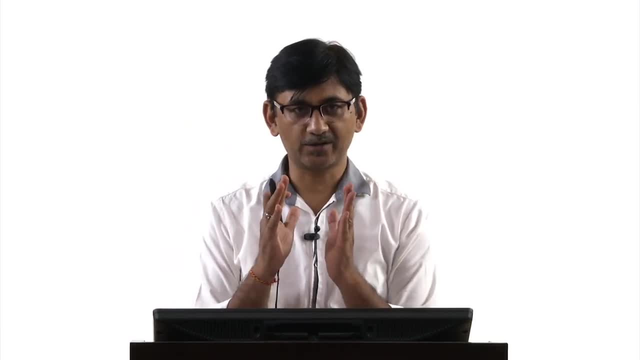 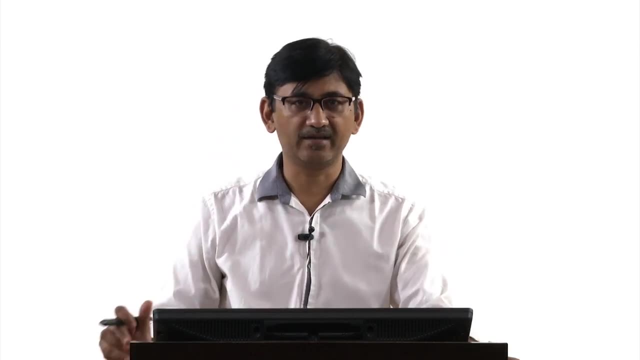 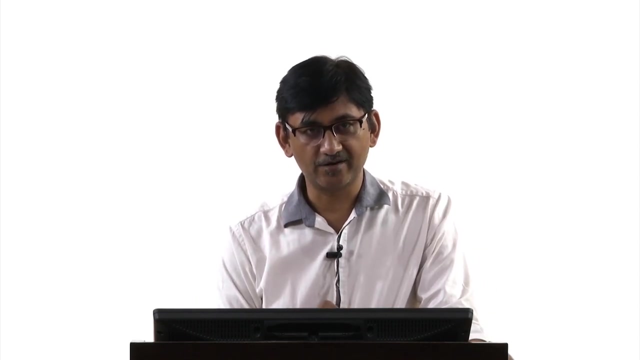 So composite. the idea of making composite is that you can combine the properties of two different material together to get enhanced property in the composites. okay, So reinforcement can be, in this case can be strong. Okay, So strong reinforcement. but it will have a problem that it can. it will be a brittle. 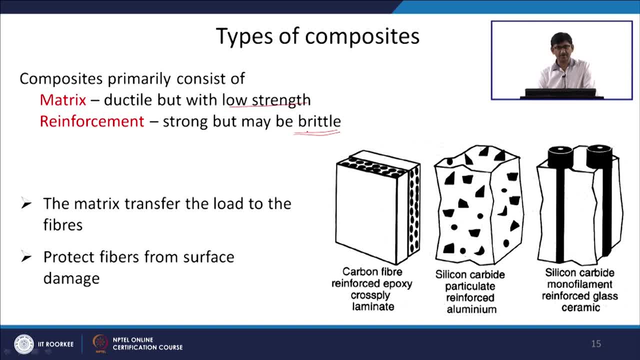 it may have a brittle nature though. it may be strong, but it may have brittle nature. So you are combining two different set of properties here. one has a ductile nature, another has a brittle nature. it has a low strength. this: these have high strength. okay. 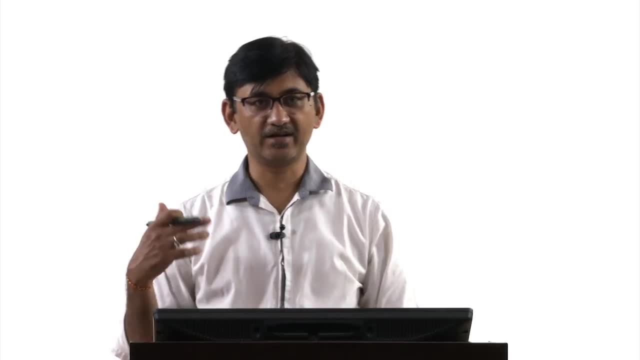 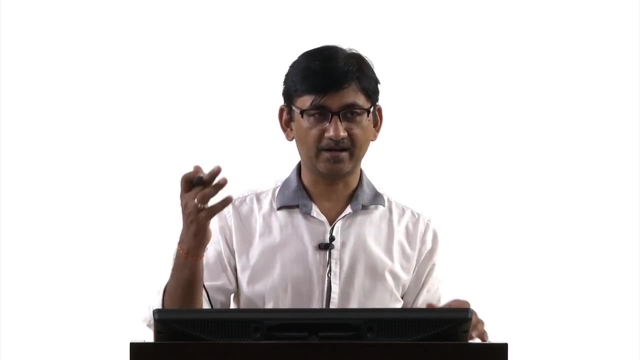 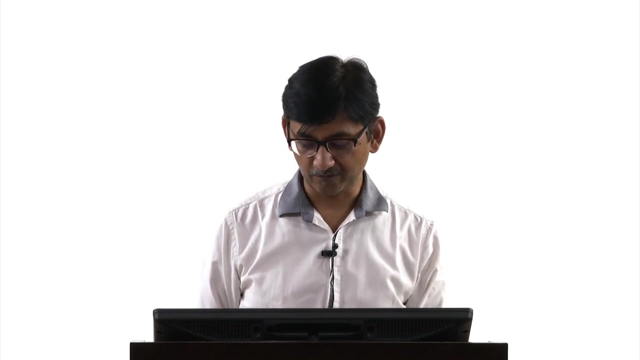 So by combining, when we have the composite, it will give you a properties which will be combination of these both and it can give you a much better mechanical properties. So there can be different type of composites. okay. For example, this one is a carbon fibre reinforced epoxy cross ply laminate. okay. 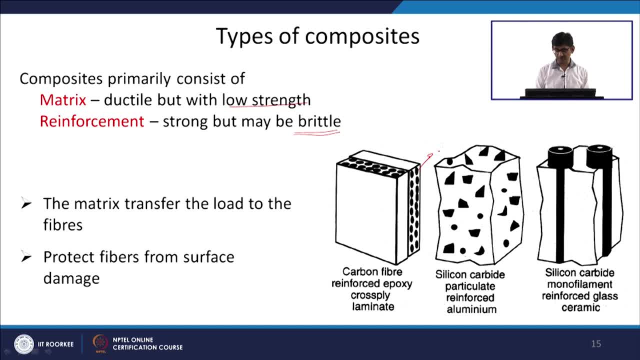 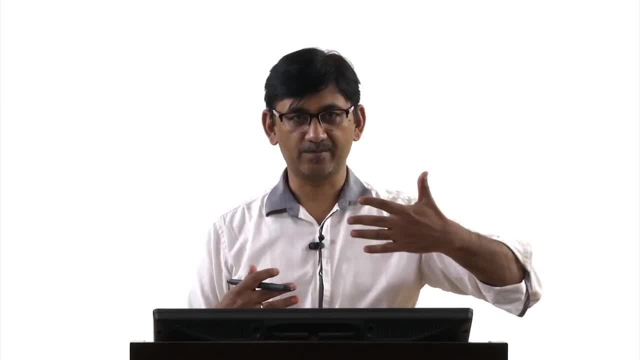 So you can see that these are the carbon fibres, okay, and they are arranged in a cross ply manner, So in one case the carbon fibre is in this direction, In another, it is in this direction. So you can see that these are the carbon fibres, okay. 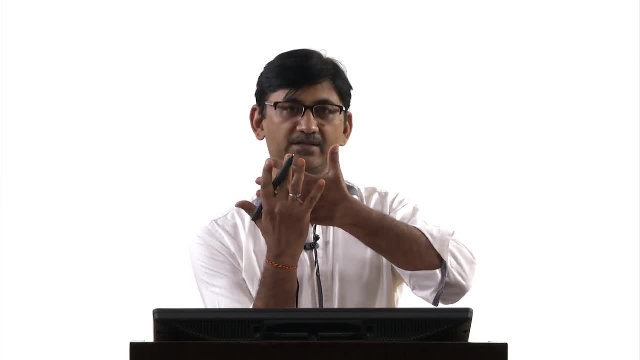 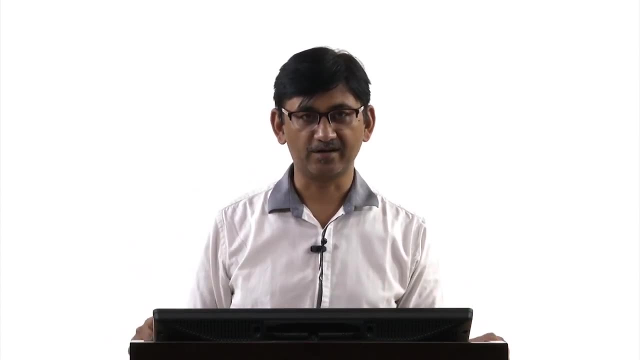 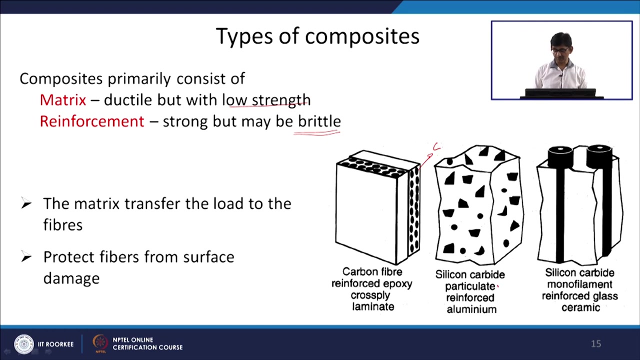 And they are arranged in a cross ply manner. In another ply, next ply, the carbon fibre is in this direction. So these are cross ply type of laminate- okay, and carbon is there for reinforcement of the matrix- okay. Similarly, there can be another type of composite which is called a particulate composite- okay. 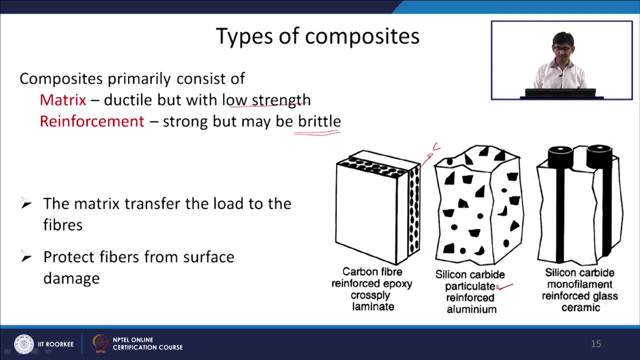 Particulate means the reinforcement is in form of particles. So these are silicon carbide particles and aluminium is reinforced with that. So aluminium is a soft material. We know that it has lower strength although very good ductility. So we are adding this silicon carbide particles in aluminium to increase the strength of the 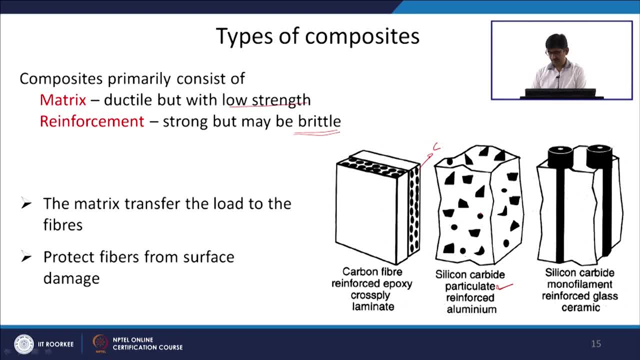 composite: okay. Then there can be this type of monofilament, reinforced glass ceramics- okay. So silicon carbide monofilaments are there? okay, In the form of this. So this is the silicon carbide, Okay, And in the matrix, okay to give to reinforce it. 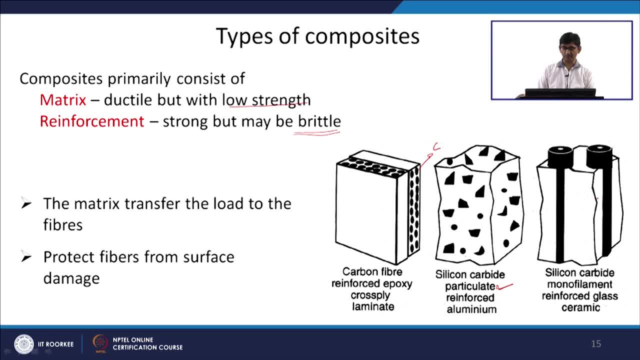 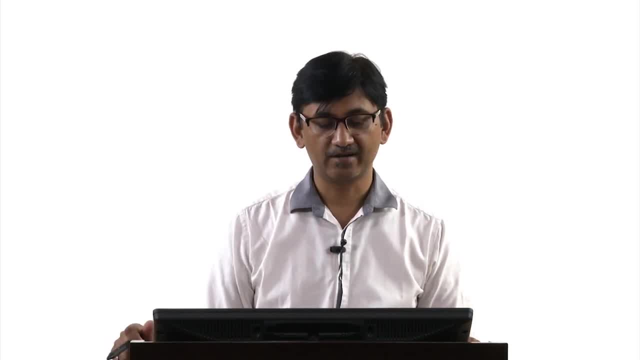 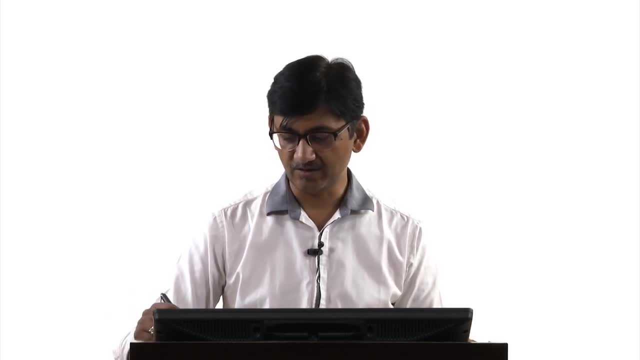 So there can be different types of ceramics possible. okay, This long fibres, maybe short fibres or maybe particulate? okay, So when we are going to discuss about mechanical property of ceramics, we will be concentrating on this long fibre, which are one of the most important composite. okay, 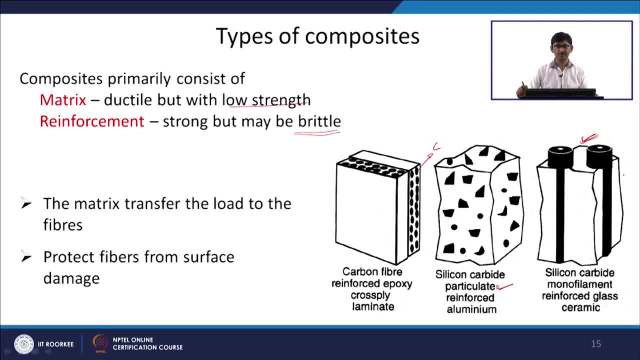 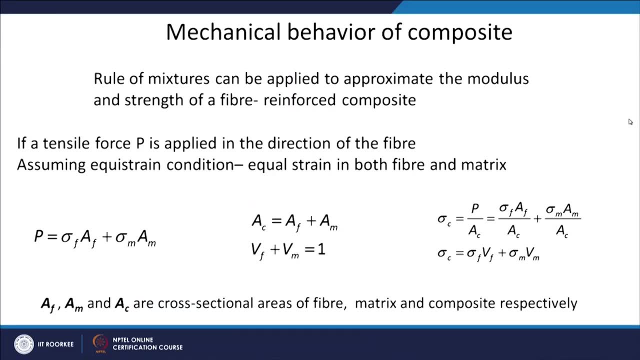 That what will be the? how you can find out the Strength and modulus properties of a composite by knowing the individual properties of the matrix and the fibre, So to find out that you can use rule of mixture. The rule of mixtures can be applied to approximate the modulus and strength of a fibre reinforced. 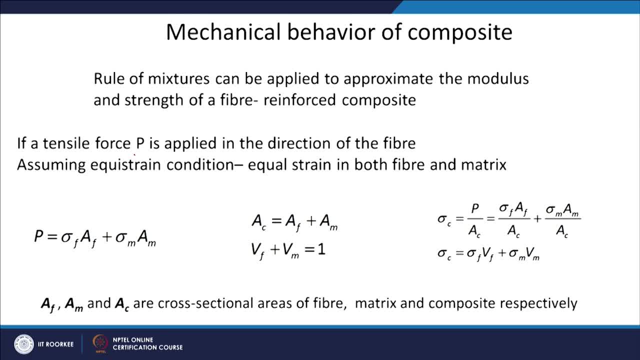 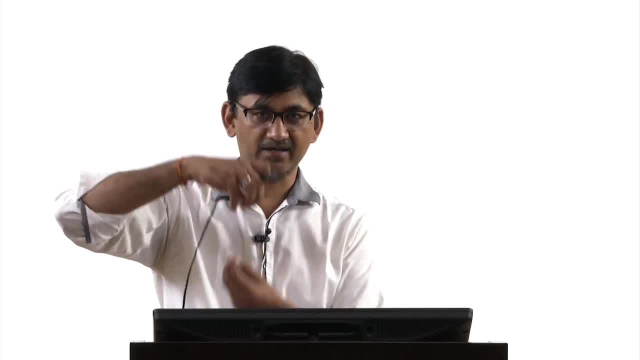 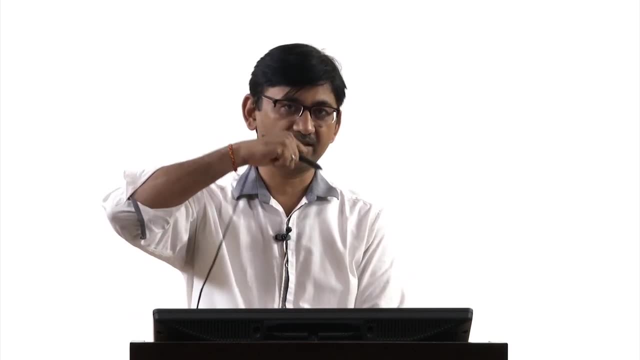 composite. So if a tensile force of P is applied, okay, in the direction of the fibre. so if fibres are arranged in this manner- Along, vertically, for example, then if I am applying the stress in the vertical direction, okay. 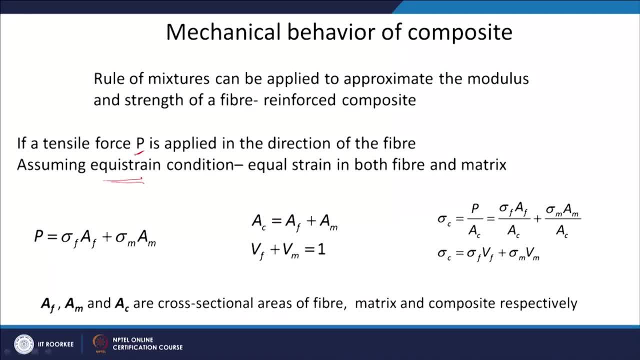 If I assume that equi-strength condition is going to be there, equi-strength mean when I am applying the force. okay, So suppose this is your matrix and in this I have fibres like this. let say I put some. 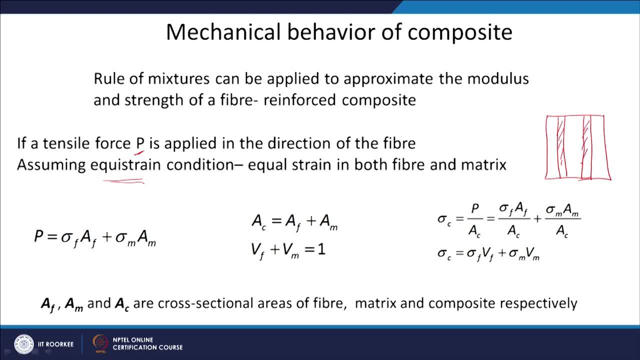 hedged And up. I am applying the stress here. okay, So some force I am applying, let say So, when these are going to deform. okay, So if there is any, there are no defects between the, between the or. there is no introduction. 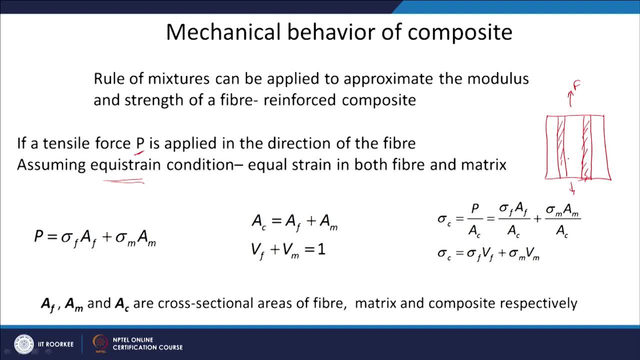 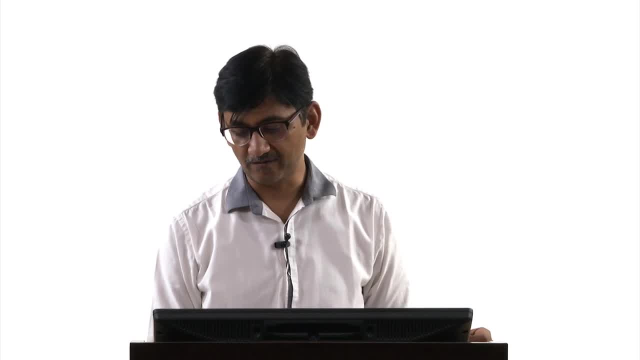 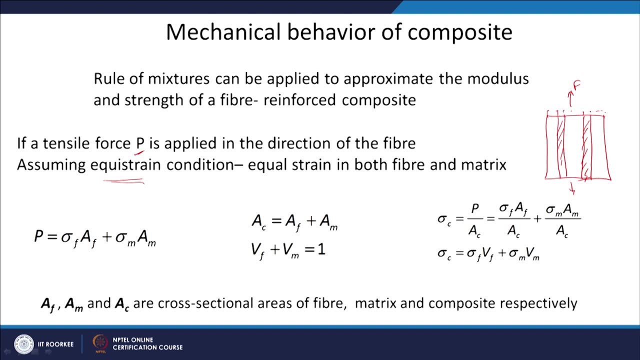 of defect between the fibre and the matrix and you have a very good bonding of fibre and matrix. what will happen? both have to deform simultaneously, okay? So after some time, Suppose time, suppose it be formed to this much dimension. okay, so it gets elongated in this direction. 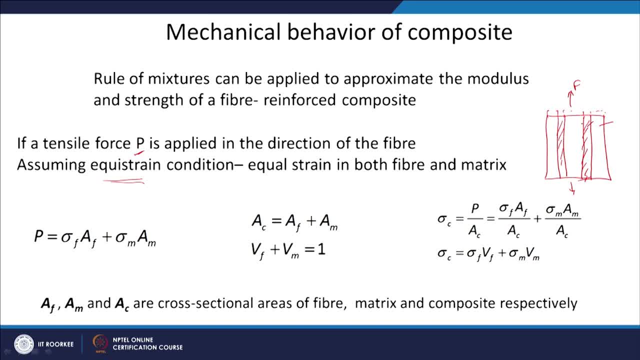 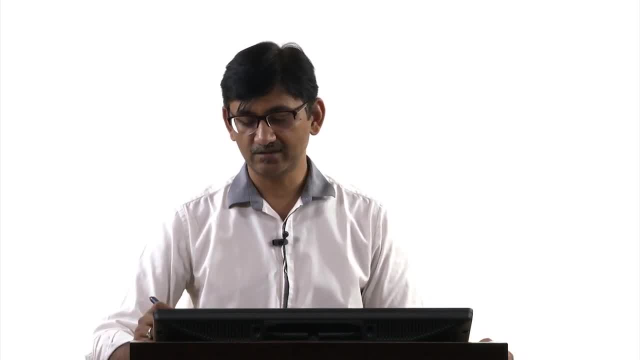 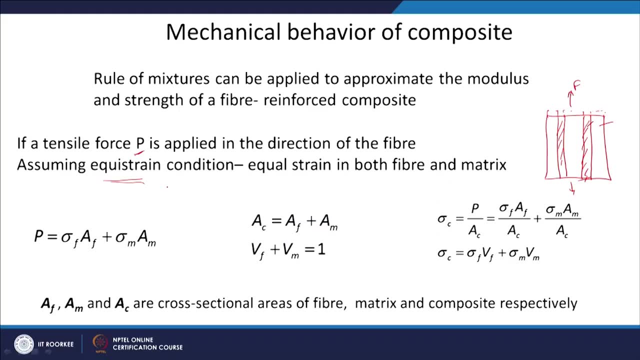 then the strain in both the matrix and the fibre will be has to be same. okay, if I am applying a stress like this, so this is a condition called equistrain condition, so in both the constituents the strain is same. okay, so basically what we are trying to say. 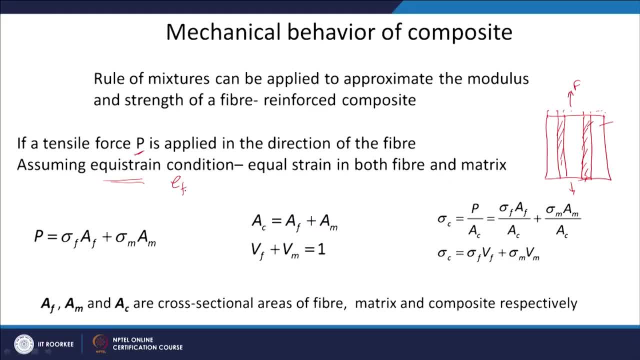 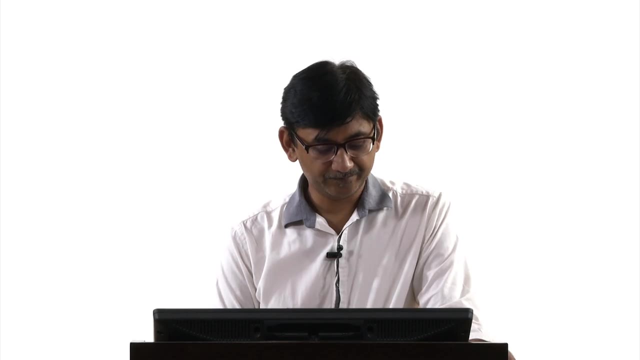 here is that strain in F, the fibre, is equal to strain in the M, which is matrix, and that is the strain in the composite. so all the 3 cases the strain is going to be same. if that is so, then I can use a rule of mixture kind of condition here that the force P can. 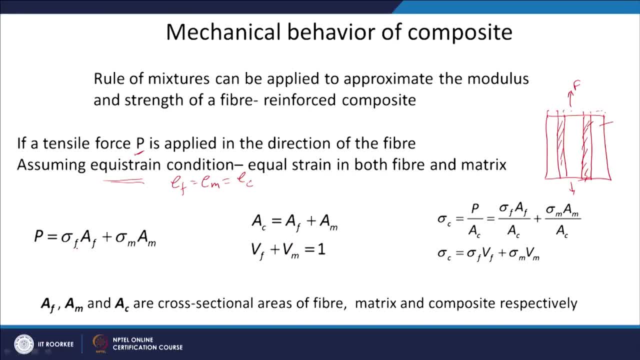 be divided between the fibre And the matrix in this form. so sigma F is the stress acting in the fibre. if I multiplied by the area of the fibre, okay, that will give me the force of in the fibre and similarly, this is the stress in the matrix. this is the area of the matrix if I multiply by that. 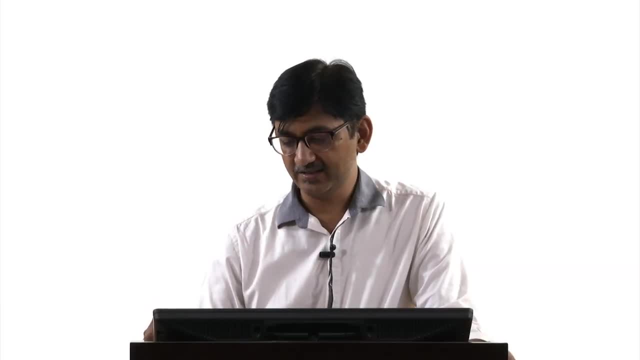 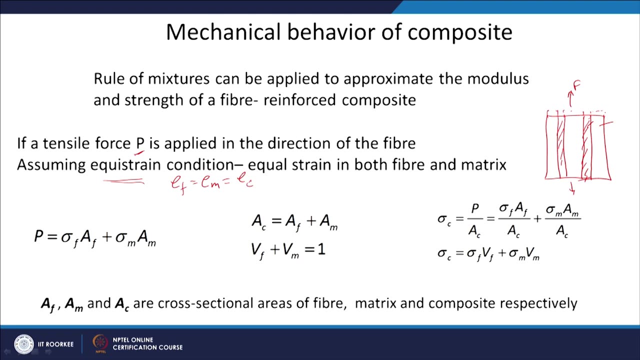 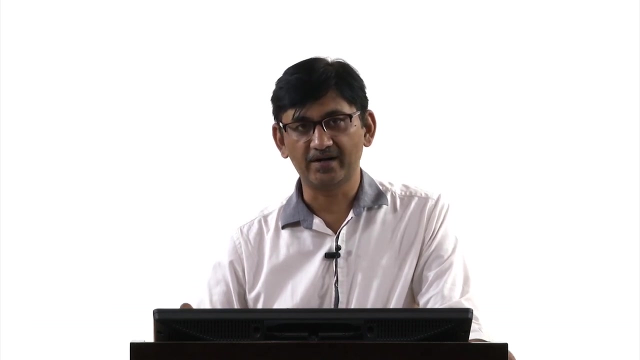 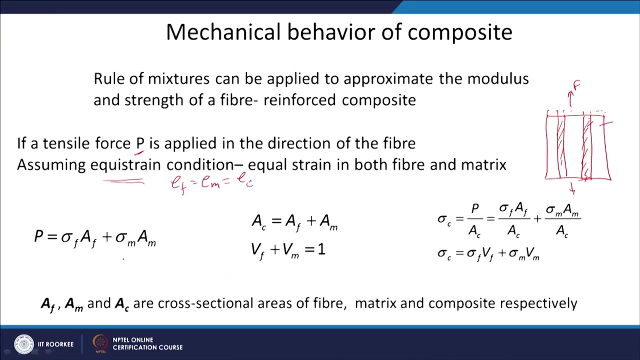 then I will get the force in the matrix. so when we are saying that this equistrain condition will be there, okay, so force will be divided between the matrix. So I can write an equation like this to express the force, total force on the system. now 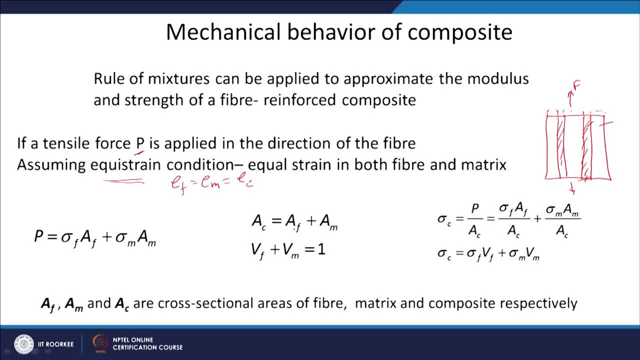 AC, the area of the composite will be basically area of the fibre plus area of the matrix. okay, And in terms of volume fraction, if you want to see, I can say that the volume fraction of fibre plus volume fraction of the matrix will be equal to 1,. 1 means it will be the 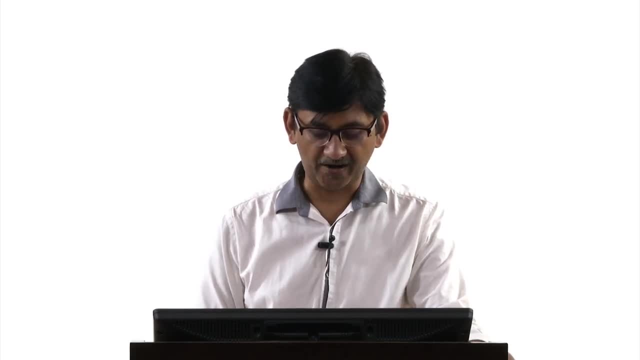 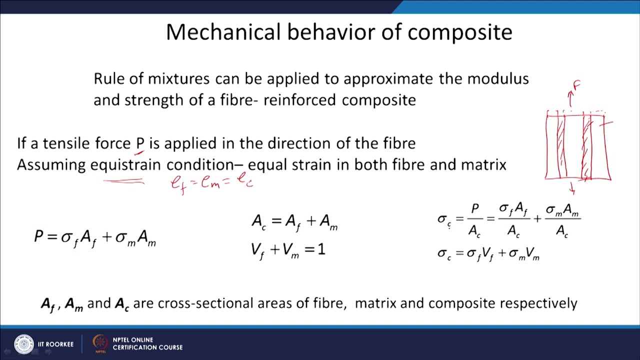 total volume. okay, so in terms of fraction, if you want to see, it will be equal to 1, so I can express this stress system here. so if I divide P by the area of the composite, then I will get the stress on the composite. 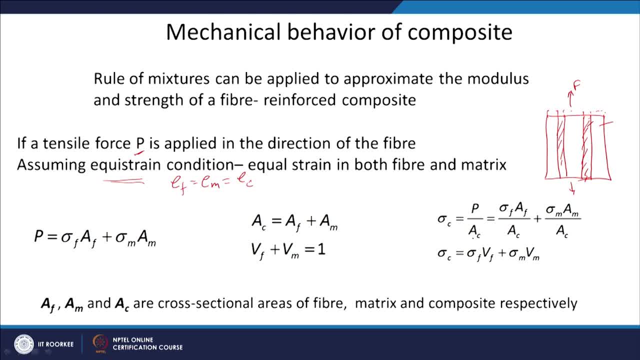 So this will be sigma C equal to P by area of the composite, which is equal to, as equation suggest here, sigma F, AF upon area of the composite, plus sigma M into AM upon area of the composite. Now the area of the fibre divided by area of the composite. okay, if you remember again, 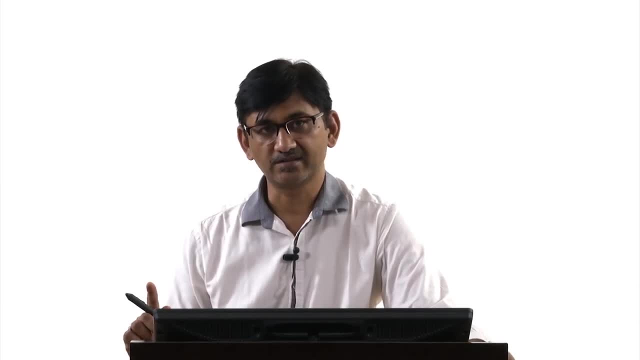 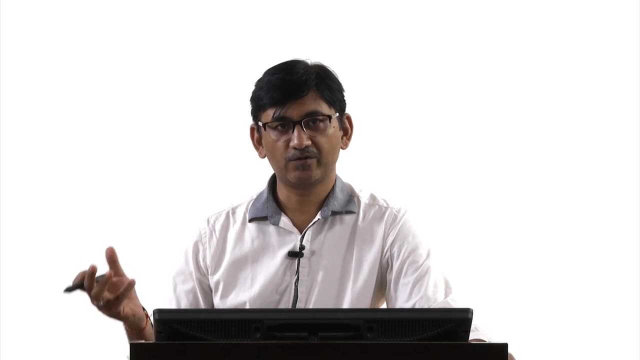 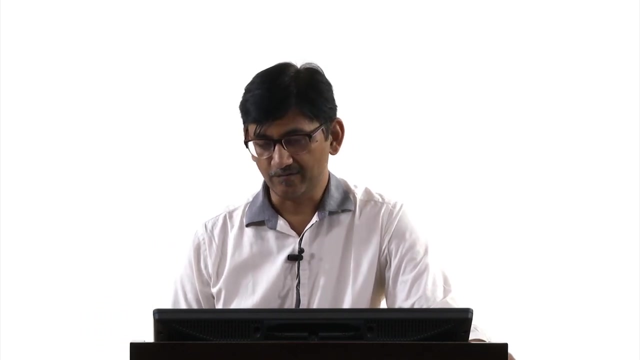 our, the one of the lecture where we were discussing about quantitative metallography, That the volume fraction, whatever you get in the area in terms of area fraction, can be considered as the volume fraction. okay, from statistical analysis. so area of fibre. 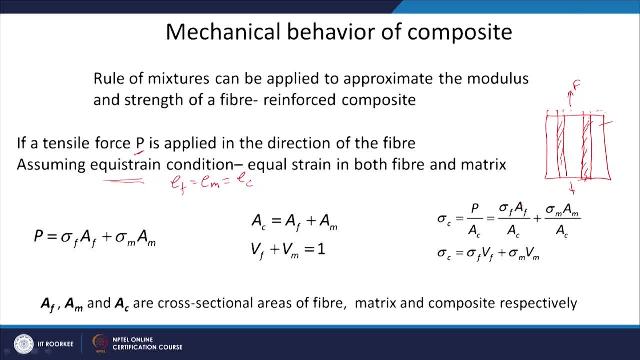 divided by total area of the composite. okay, will give me the fraction in area, okay, And that I can say that it will be also as fraction in volume, okay, so this will be now. sigma F into F by AC will be written as VF here, and AM by AC will be written as: 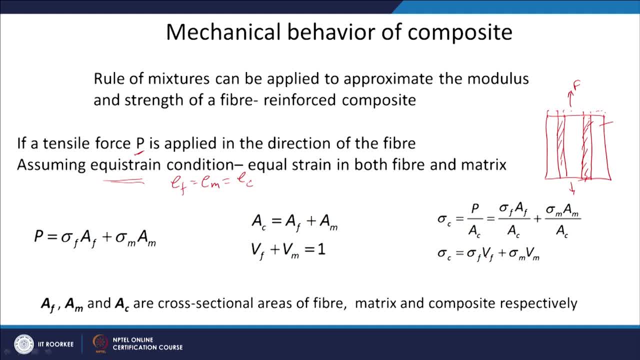 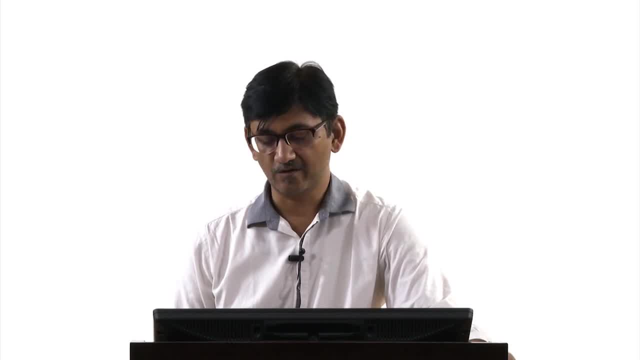 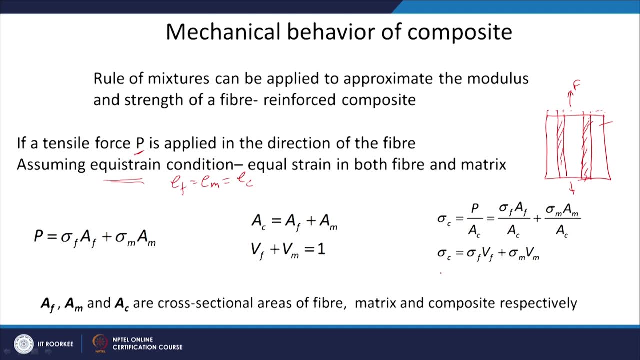 VM here. so this is volume fraction of matrix, this is volume fraction of fibres. okay, so I can write a simple rule of mixture kind of equation like this: to get the stress of the stress in the composite, You can in fact write for the modulus also. modulus of the composite will be equal to. 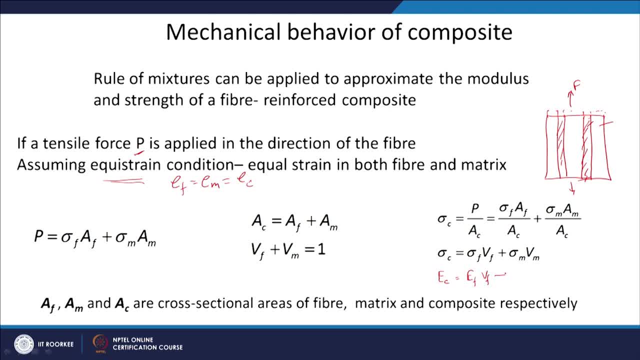 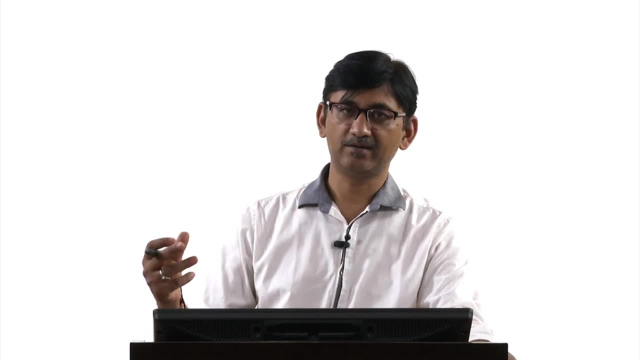 modulus of the fibre into volume fraction of the fibre, plus modulus of the matrix into the volume fraction of the matrix. okay, so I can write it for modulus also, as I am writing for stress, to get what will be the modulus of the composite. okay, so these two equations. 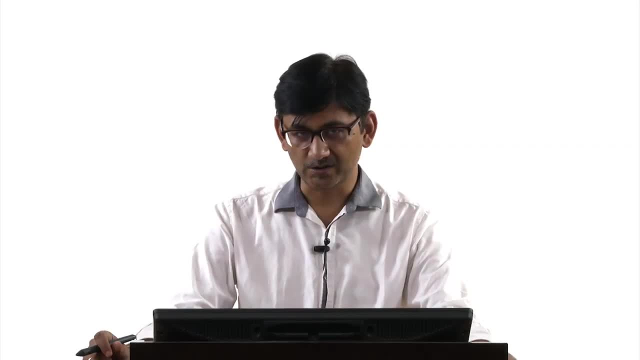 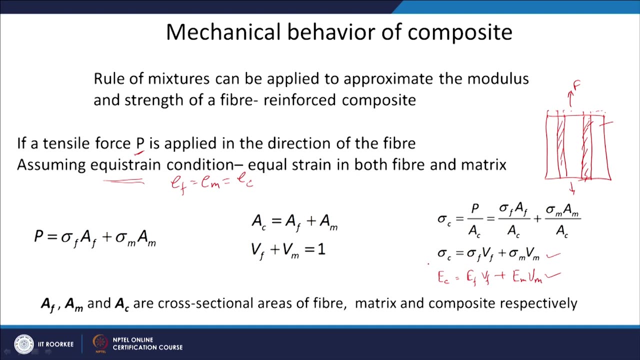 we have to kind of remember by using rule of mixture. okay, so depending upon what is the volume fraction of fibre it will have that much contribution to the total composite stress or strength and similarly, what is the volume fraction of matrix that will be contribute. 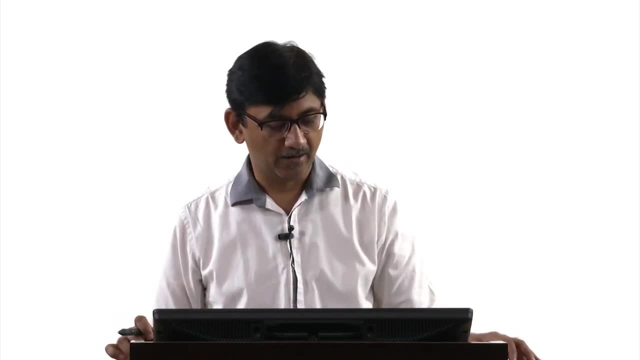 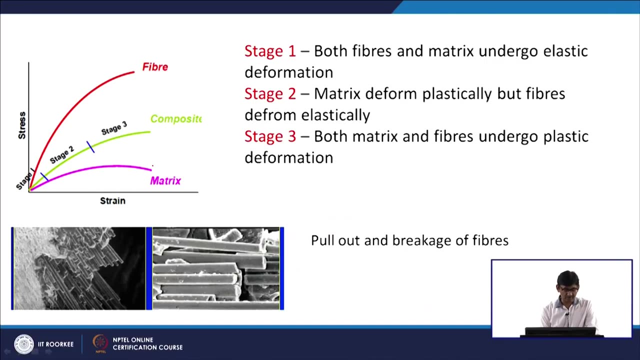 to the total strength of the composite. Now, if you want to see the stress-strength curve in terms of composites, okay. so, for example, for a matrix, the stress-strength curve is like this: okay, which is having lower strength. 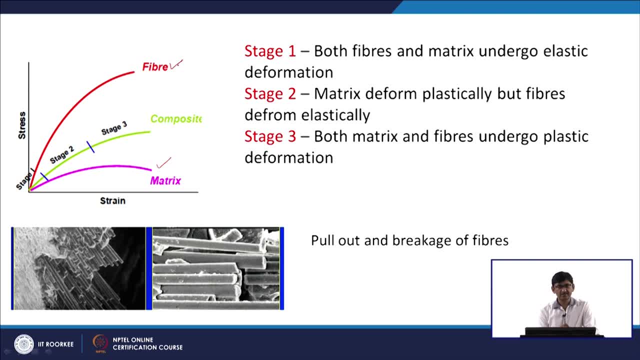 So it has higher modulus and lower modulus and so on. the fibre is very stiff. okay, it has higher modulus, higher strength and so on, but have lower ductility. so we can have a composite of these two to get strength in between the modulus of in between the 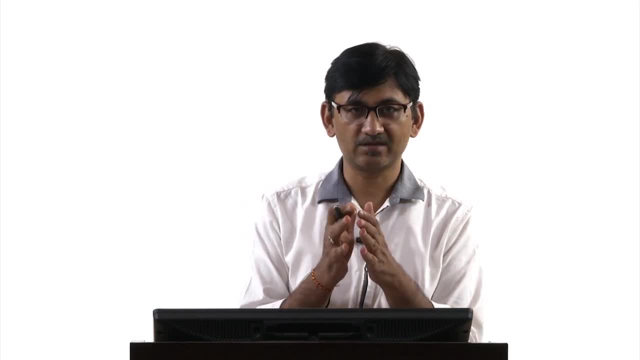 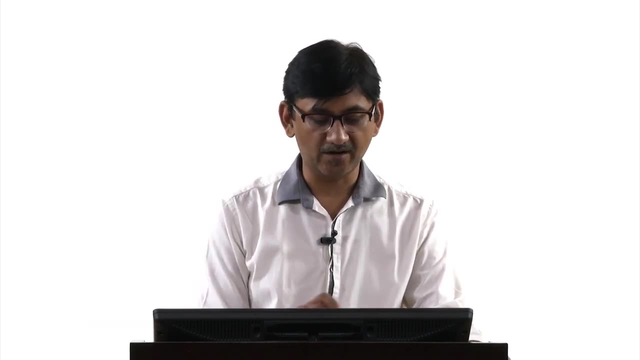 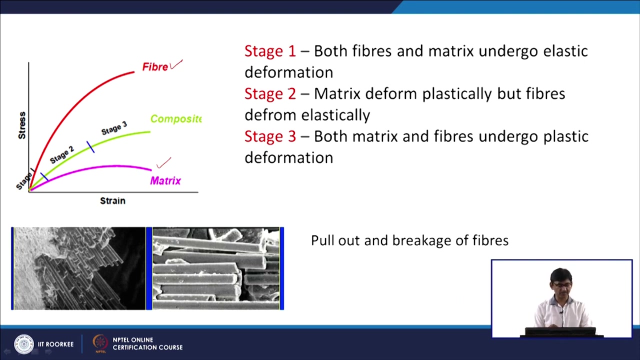 two. okay, so we get a good compromise of property between the two, the matrix and the fibre. okay. so if you see the deformation of the composite, it can be divided into three stages. So in stage 1, both fibre and matrix undergo elastic deformation. okay, up to this point. 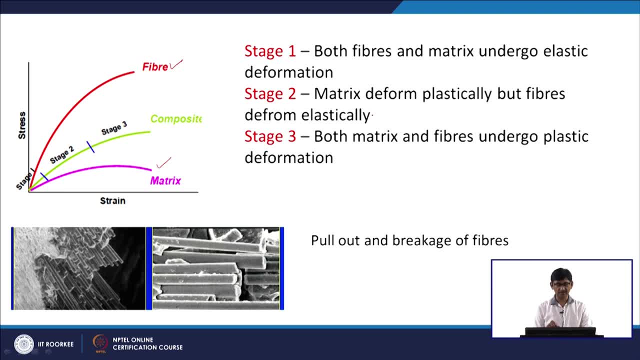 Stage 2, matrix deform plastically, but fibre deform elastically. okay. and stage 3, both matrix and fibre undergo plastic deformation. so if the fibre is not, does not exhibit any plastic deformation. for example, the fibre is made of ceramics, just for an example. and 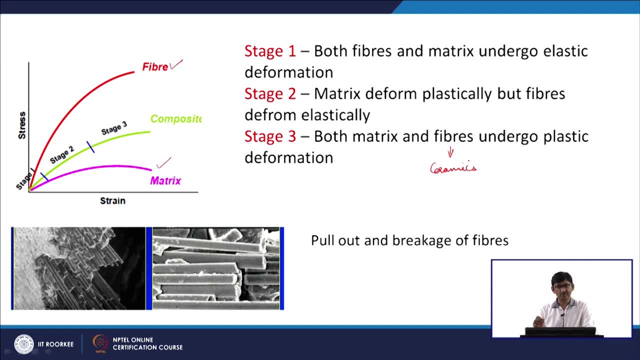 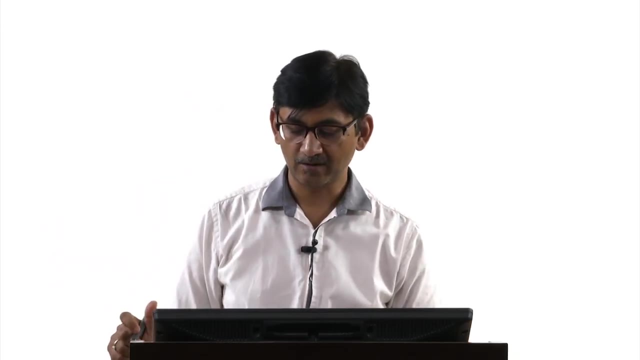 it does not show any plastic deformation, then the whole deformation, throughout the deformation of the composite. this will show only the elastic deformation- okay, whereas the material is showing the plastic deformation- okay, and we know that it will show the elastic deformation and then it will break. okay, though the matrix will keep on deforming plastically. 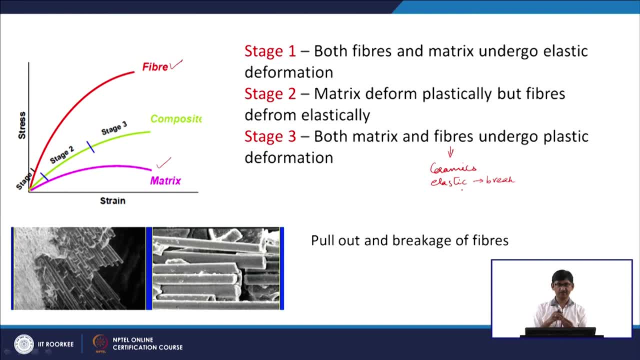 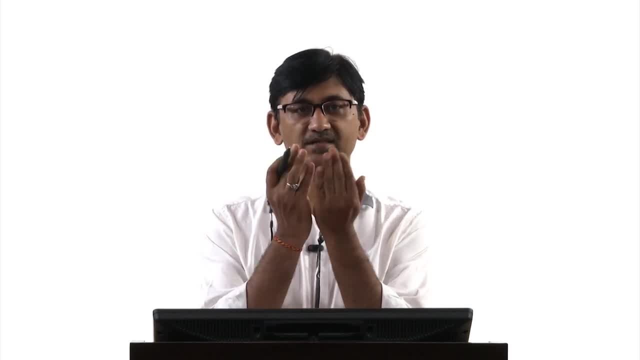 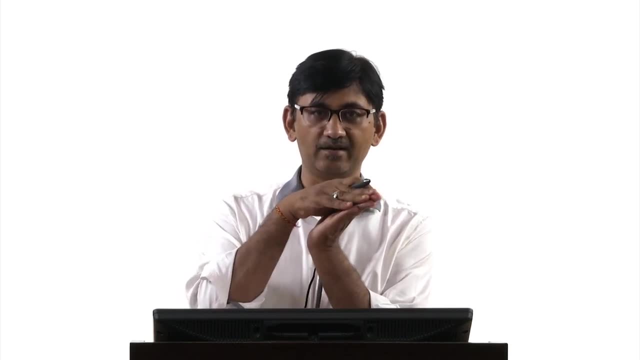 okay. so when it breaks, the crack will propagate through the plastic And through the ceramic. but because these fibres are surrounded by the matrix, the ductile matrix, this crack will not go beyond the matrix. okay, in the matrix, the crack will. 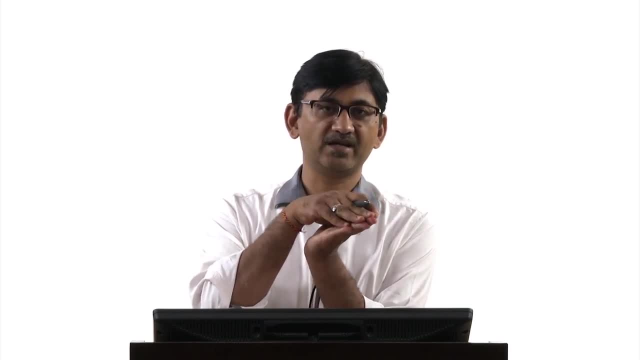 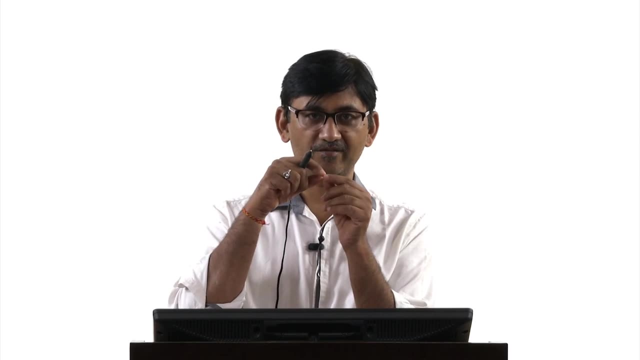 be blunted. okay, it will not be, it will not remain as sharp. so by doing this kind of making a composite, what we are doing is that the, if any because of defect, any one fibre breaks. also, the crack is not propagating through. Throughout the material. If the whole material is of ceramic, what will happen if a crack start propagating, it will propagate throughout the volume of the ceramic and the whole material will fracture. By making a composite what we are doing is, if any one fibre breaks because of any defect, 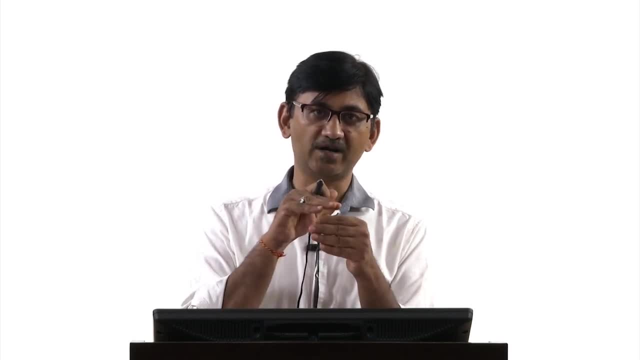 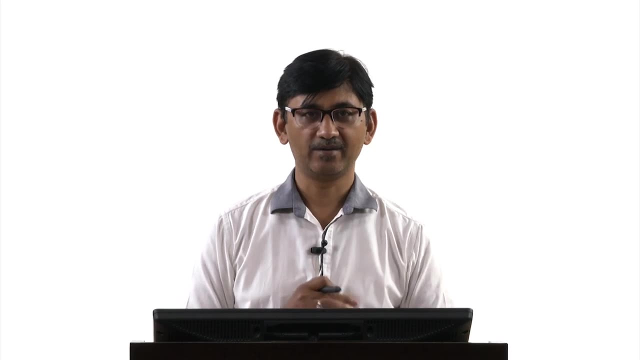 in that, okay, the crack will be limited only to that fibre. only that fibre will break and it will not. the crack will not propagate beyond that fibre. And around that fibre there is a ductile matrix. okay, so if you keep on deforming, 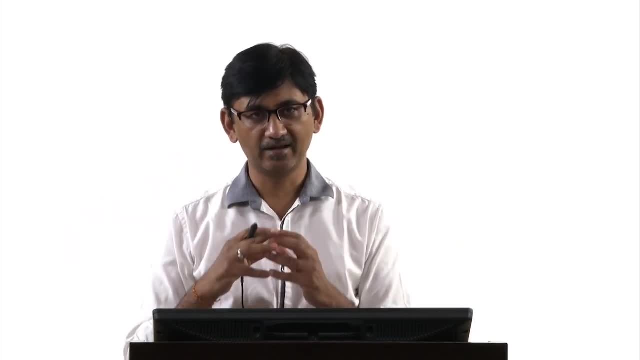 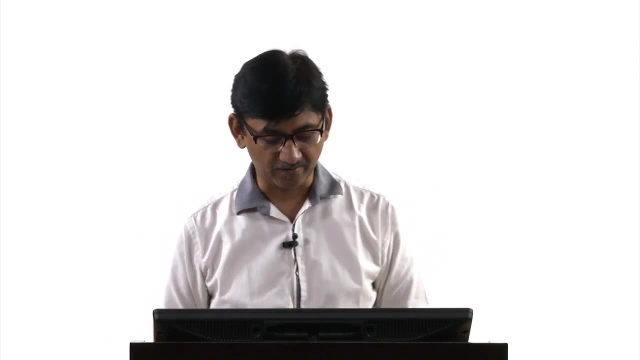 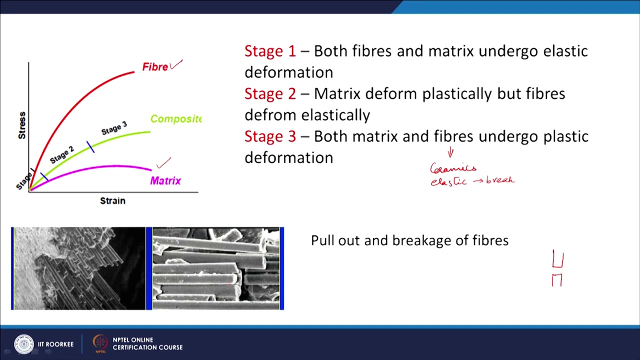 the material and all the fibres will keep on breaking and the remaining material will deform plastically. what you will see after the deformation: if you do the analysis of the fracture sample, you can see that these fibres are broken in a brittle manner with.